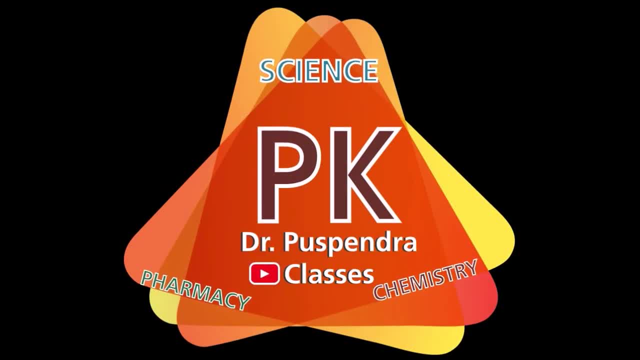 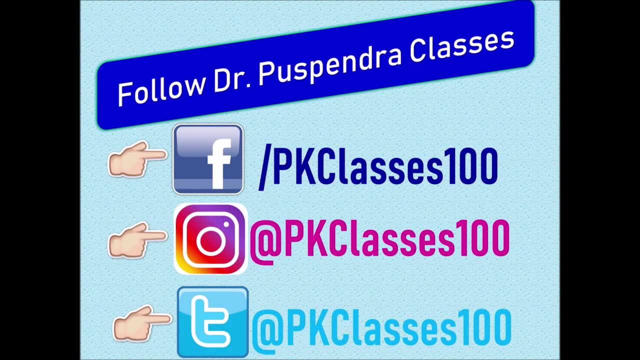 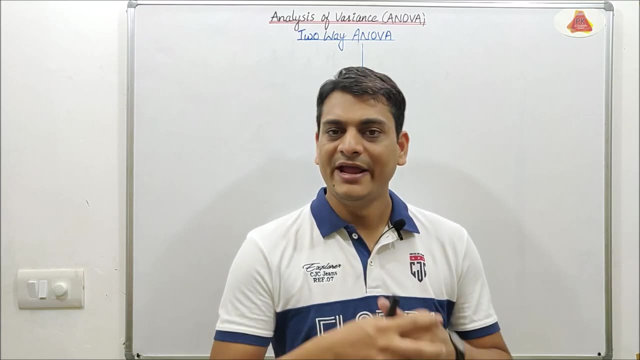 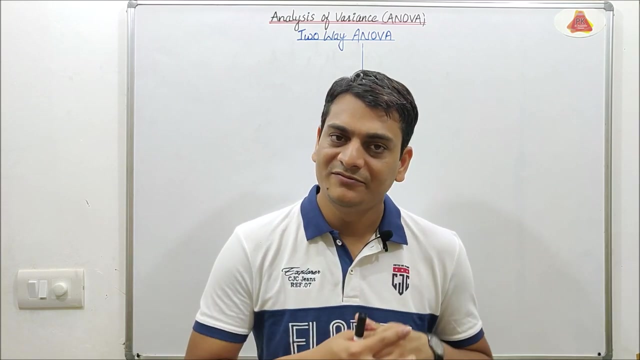 Hello friends, today I am going to discuss about two-way ANOVA under analysis of variance. But before watching this video, I will strongly recommend you to watch my previous videos on ANOVA. Link of those videos are given in the description. 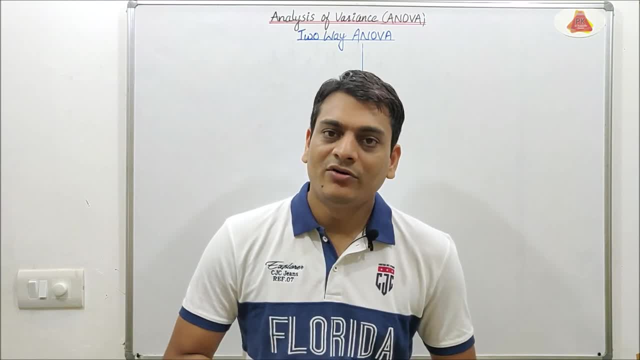 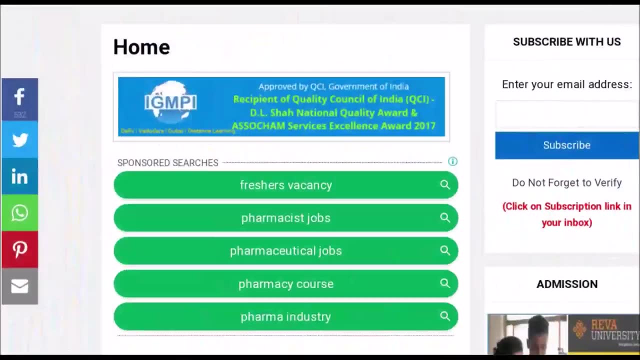 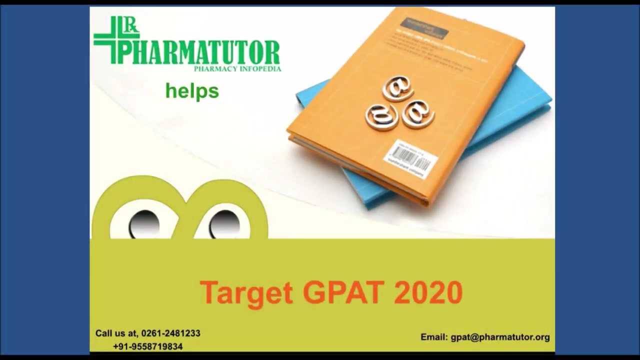 Now coming to two-way ANOVA, So it is classified according to two factors or two criteria. This video is sponsored by PharmaTutor. They provide job alerts, pharma newsletters, admission alerts, articles and many more. You can also join online test series for GPI. 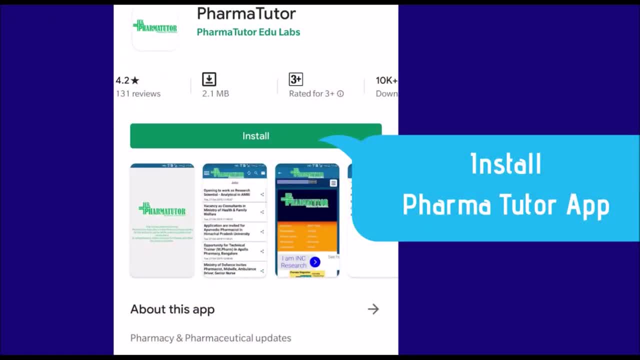 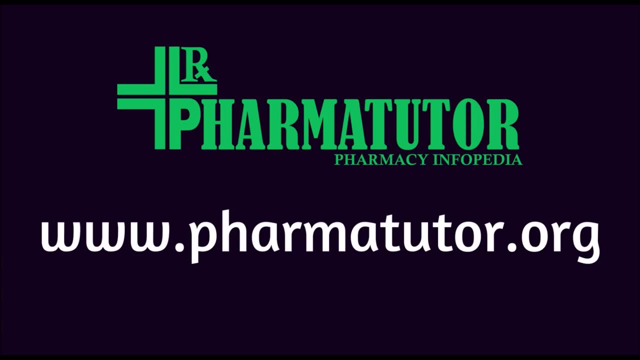 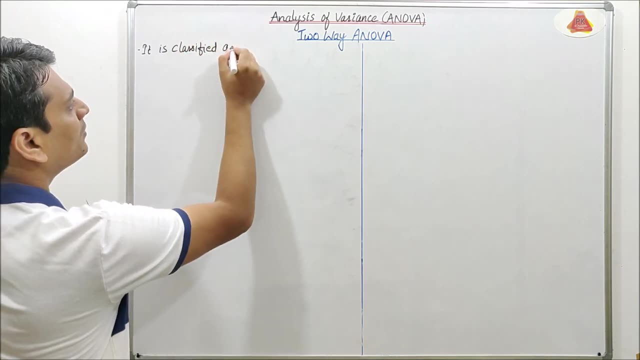 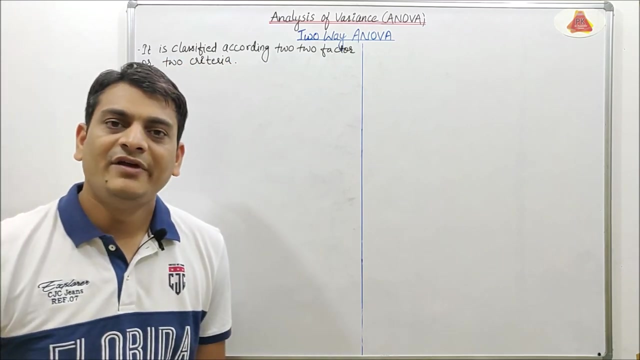 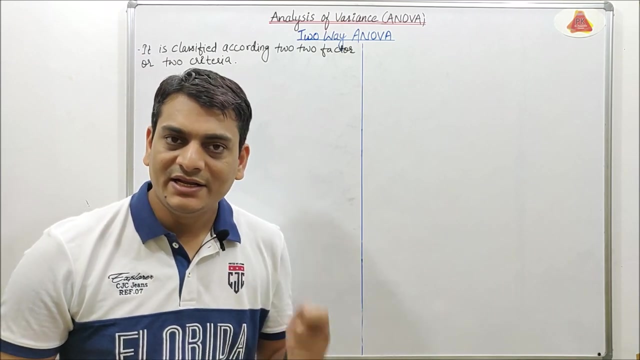 preparation. Download dedicated PharmaTutor app for regular notifications. Visit wwwpharmatutororg for more details. Link is given in the description. As you know, one-way ANOVA is classified according to only one criteria, But here two criteria are present. So let's take an example for 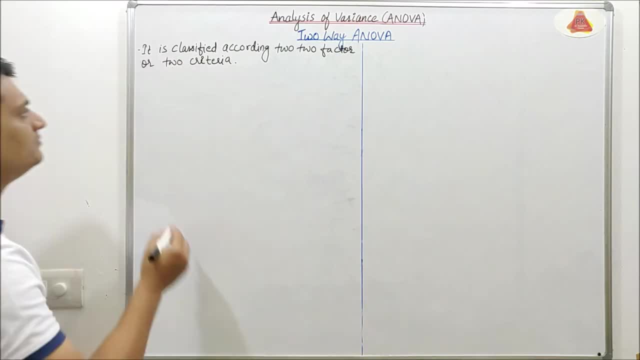 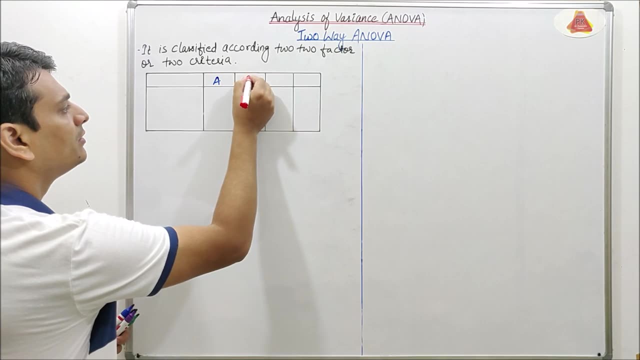 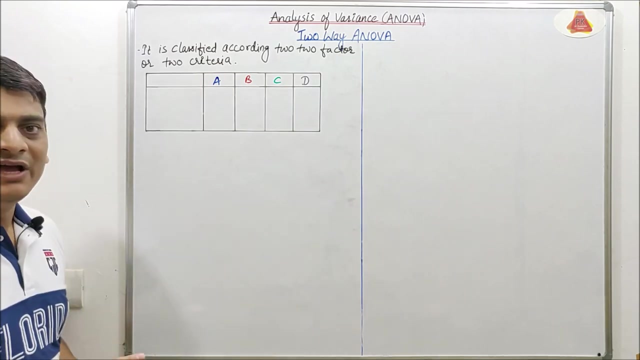 better understanding the concept of two-way ANOVA. So, for example, we are having four students Which are A, B, C and D And we are observing their study hours in three days, which are Monday, Tuesday and Wednesday. So Monday is denoted by M, Tuesday is denoted by T, Wednesday is denoted by W, For example. 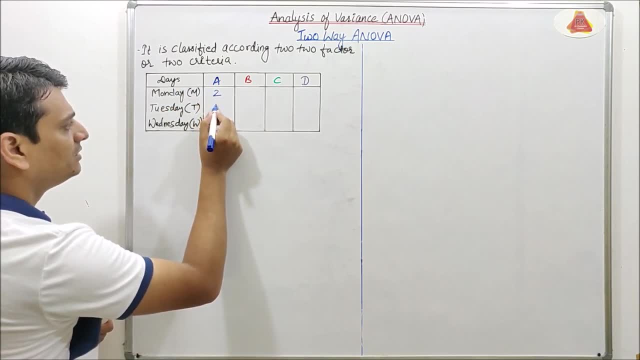 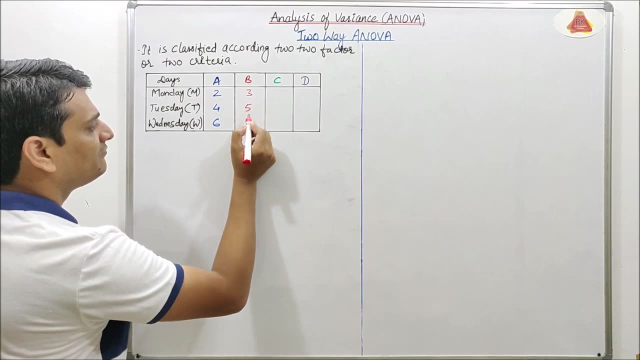 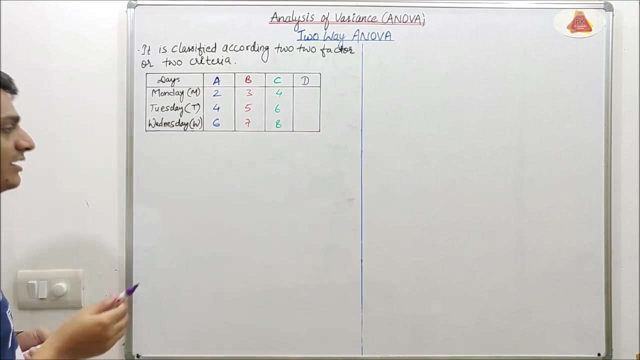 A studied on Monday for two hours, then four hours, then six hours. Let's take the B, So it is three, five and seven hours. Let's take the C, So it is four, six and eight hours. Let's take the D, So it is five, seven and nine hours. 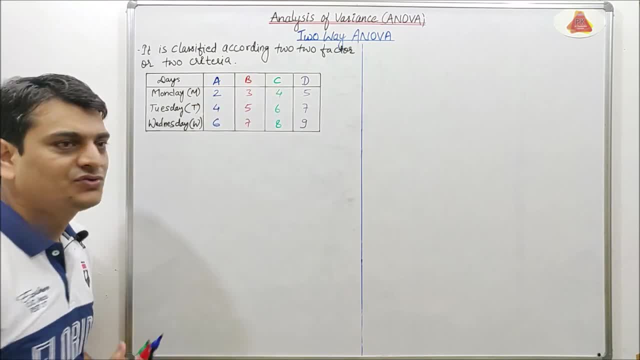 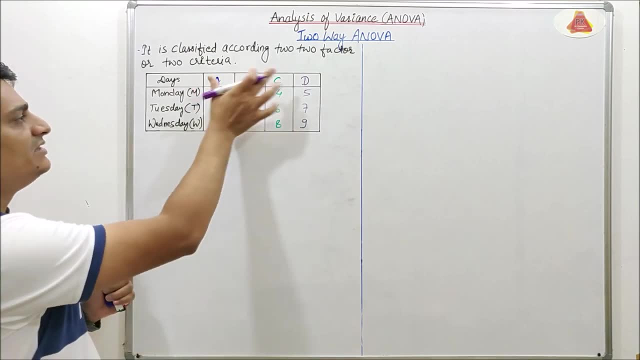 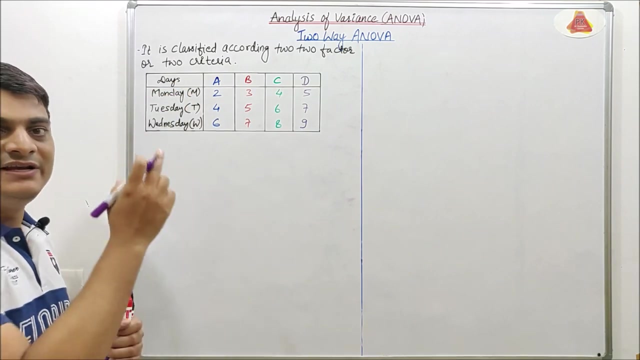 Now we will apply two-way ANOVA in this given data, So we can define two criteria. First one is: variance between the columns means variance between these four students, that is, A, B, C and D. Second one is variance between these days means variance between the rows. 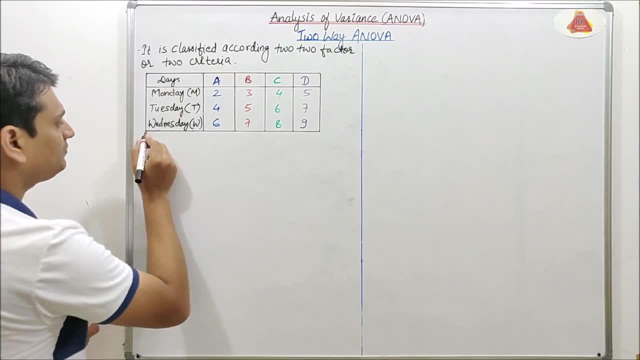 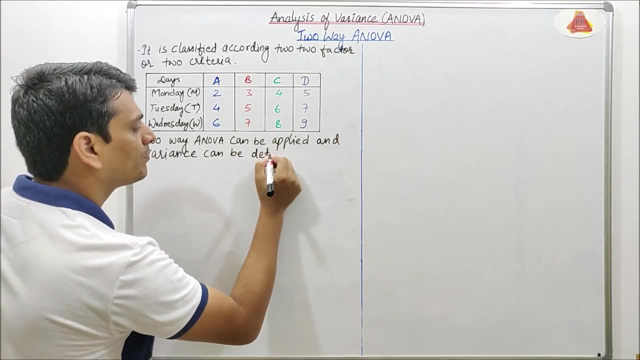 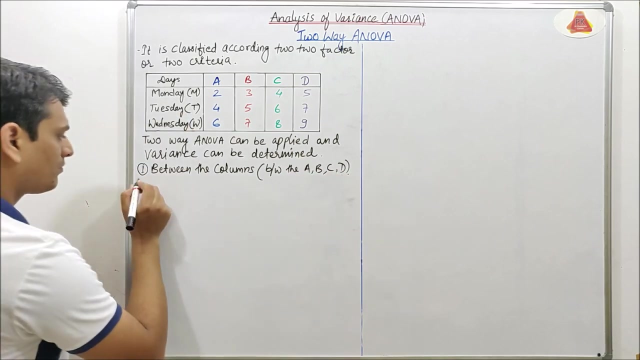 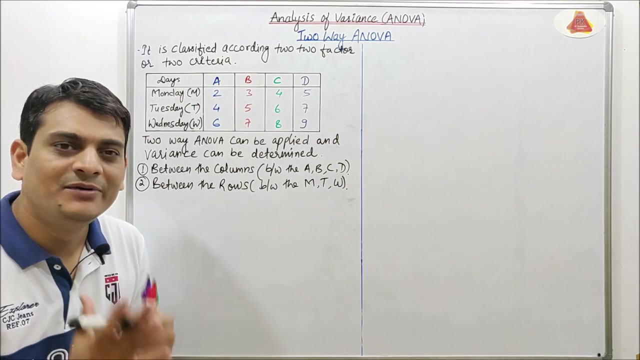 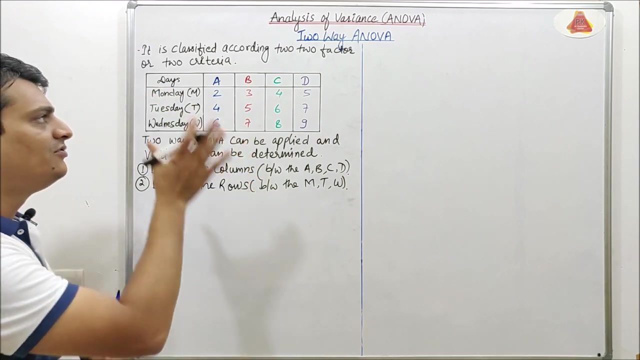 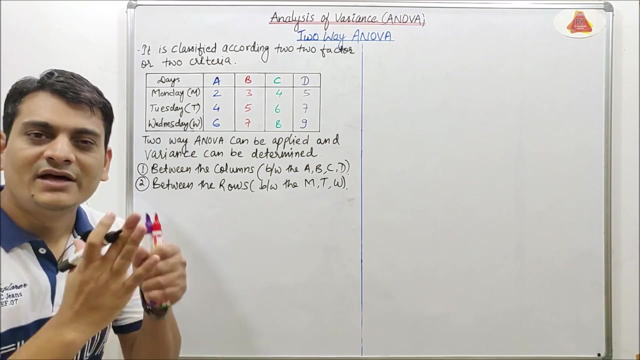 which are Monday, Tuesday and Wednesday. So here two independent variables are present, which is between the students and second one is between the days. That is why here we will apply two-way ANOVA to determine the variation between the students and a variation between the days, And these are two criteria. So 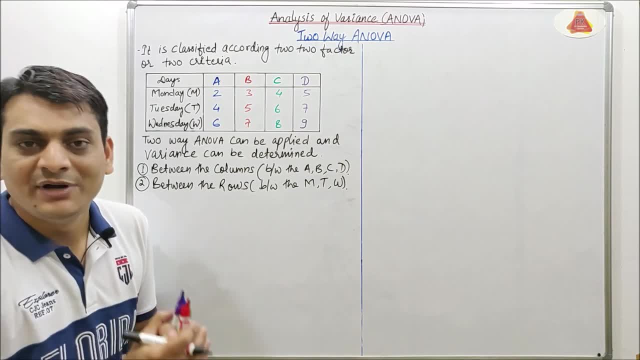 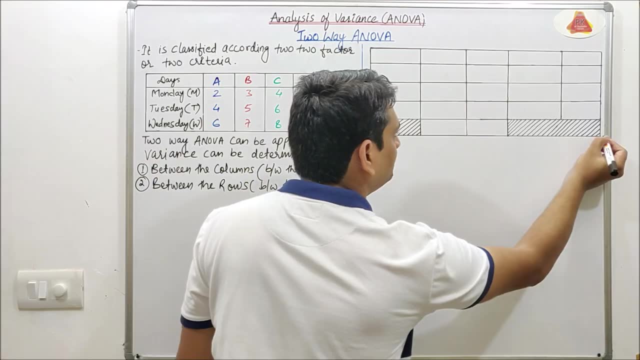 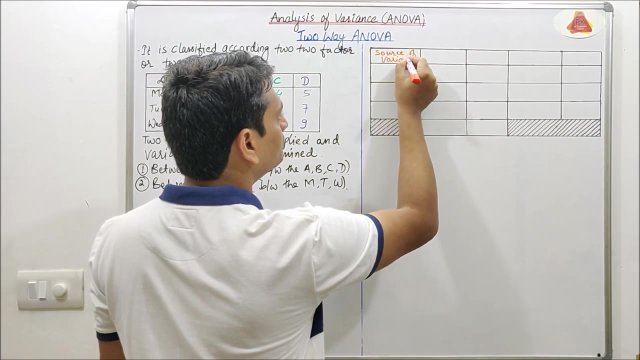 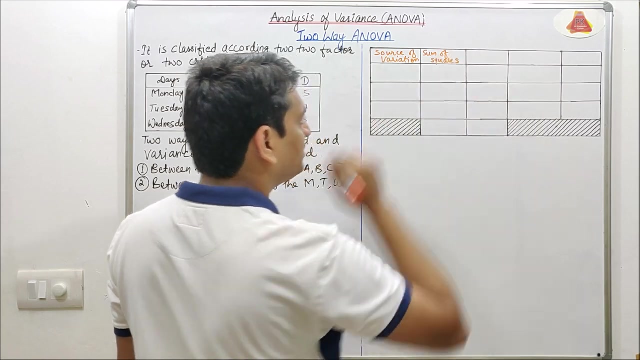 just like one-way ANOVA. here also we are having a table to calculate the F value for two-way ANOVA And the table will be like this. So this is the table, and the first column is for source of variation. Second column is for sum of squares. Third column is for degree of freedom. 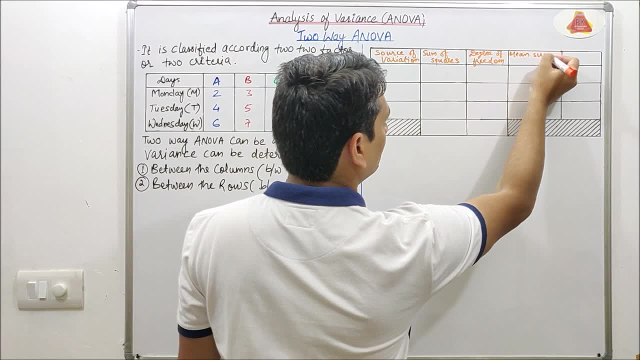 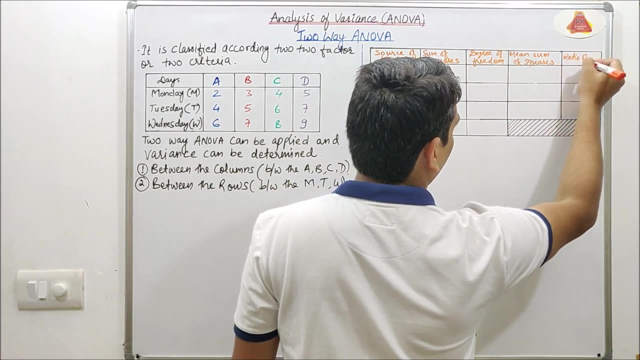 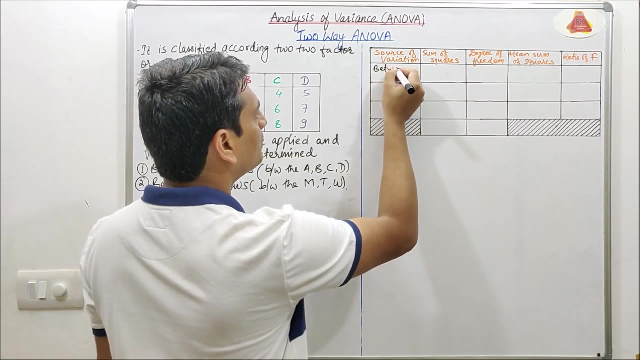 Fourth column is for mean sum of squares. The last column is for ratio of F. Now coming to the first column, that is source of variation. So it will be between the columns. So sum of square between the columns is denoted by: 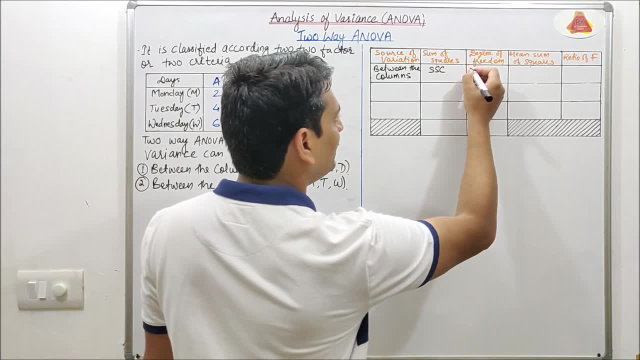 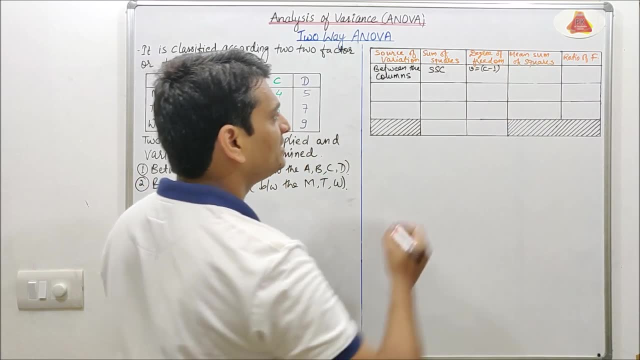 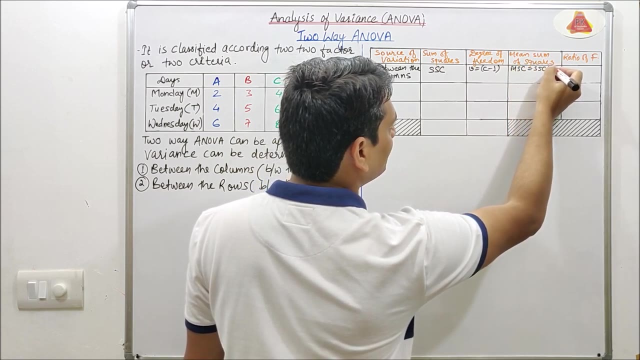 S, S C. Degree of freedom is denoted by nu, So nu is equal to C minus one. Mean sum of square is denoted by M S CAPTIONS FOR Early program ofkyetik yahoodチي. and msc is equal to ssc divided by c minus 1, and the ratio of f for between the columns is denoted: 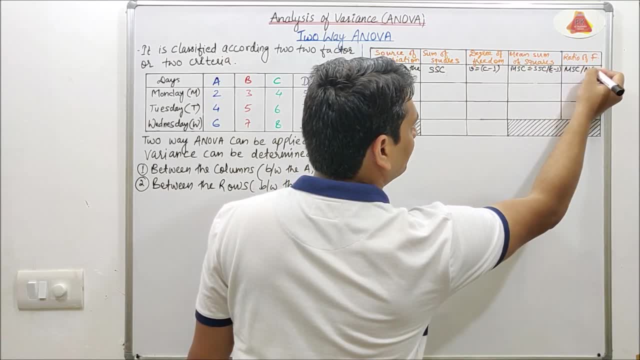 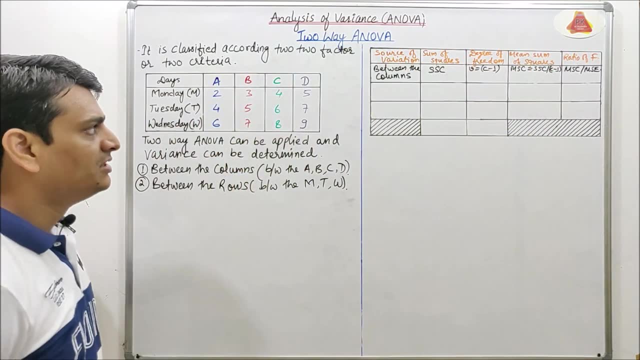 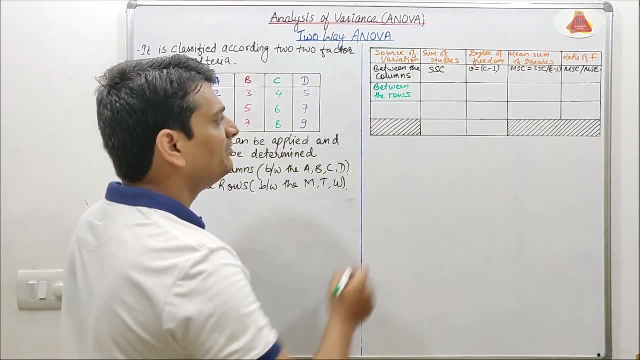 by msc divided by mse. so this complete row is for calculation of between the columns means this is the between the columns now coming to between the rows. so sum of square between the rows is denoted by ssr, degree of freedom is denoted by nu, is equal to: 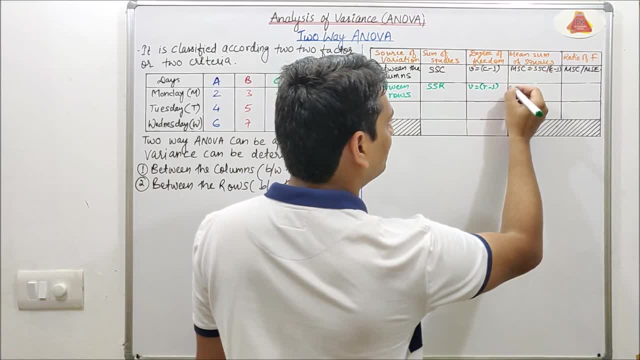 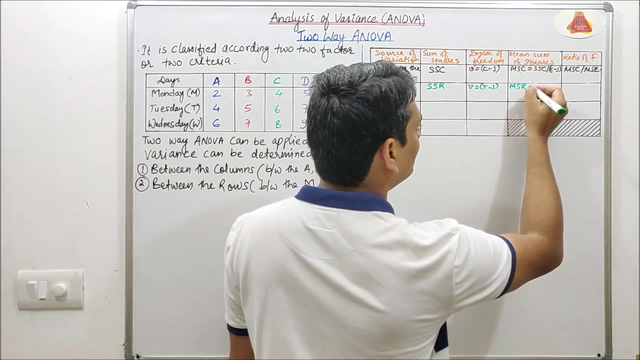 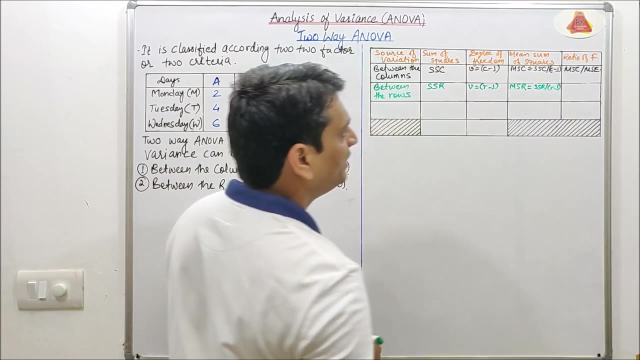 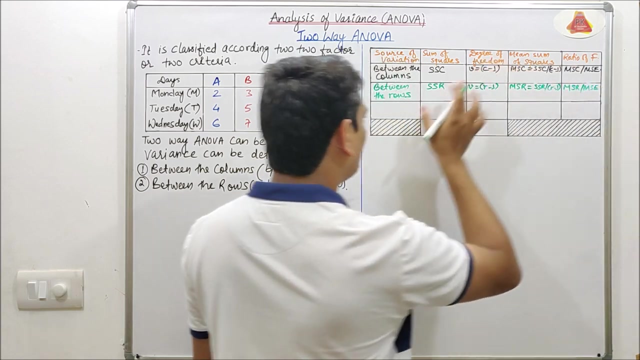 r minus 1 mean sum of square is denoted by msr, and msr represents to the mean sum of square between the rows, and the formula will be ssr divided by r minus 1 and the ratio of f will be MSR divided by MSE. Now coming to the third row, which is for residual or for errors, 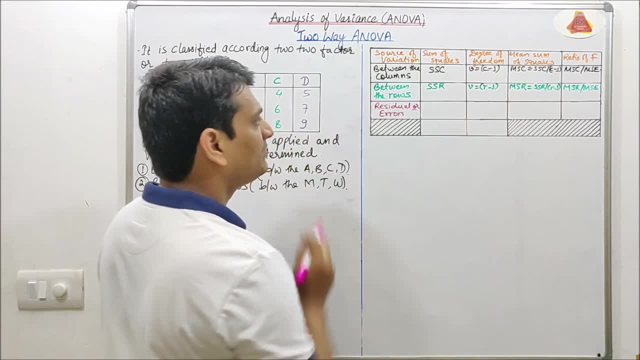 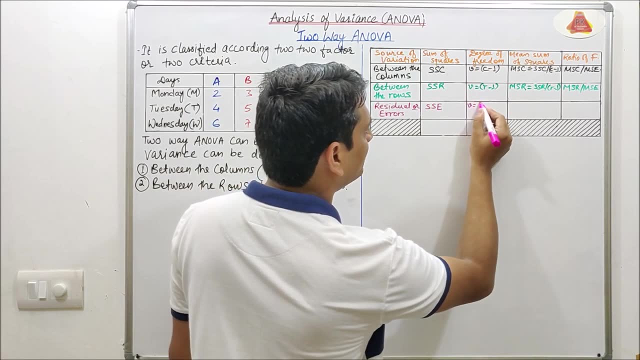 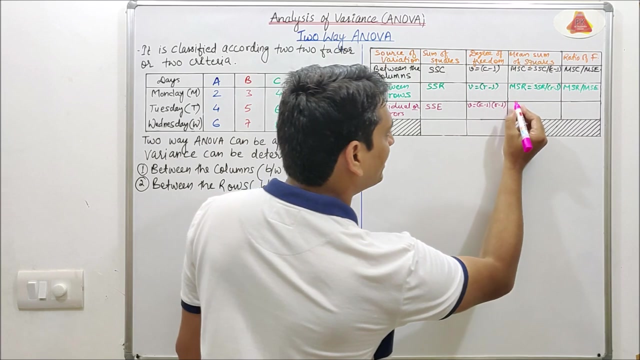 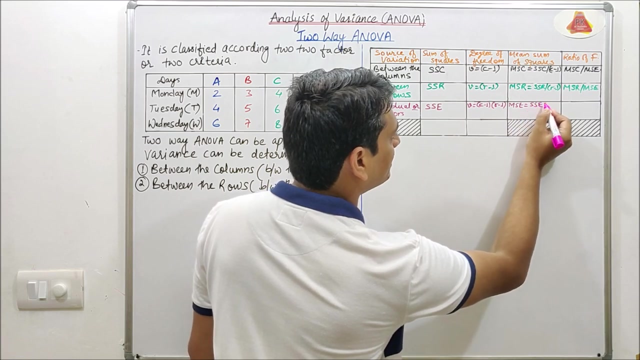 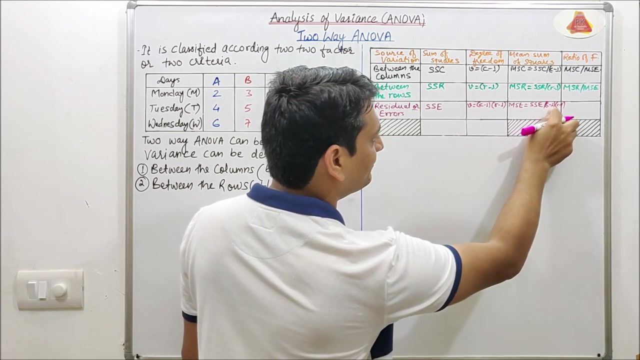 so sum of square due to error is denoted by SSE. degree of freedom nu is denoted by C minus 1 into R minus 1, and the mean sum of square due to error is denoted by MSE, and MSE is equal to SSE divided by this C minus 1 into R minus 1. this is degree of freedom, and here we will use SST. 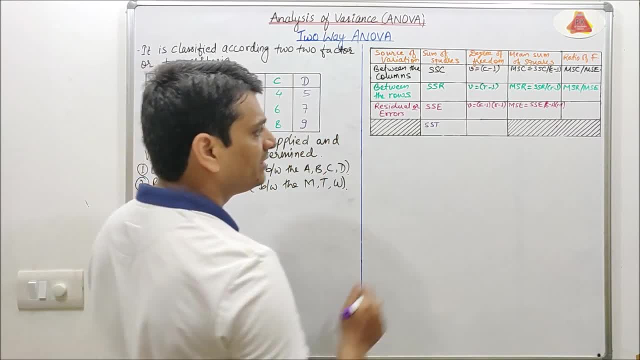 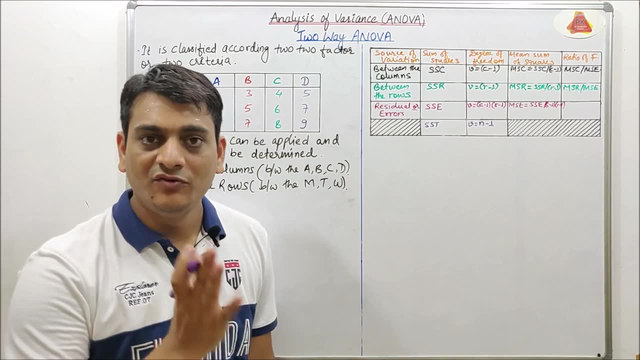 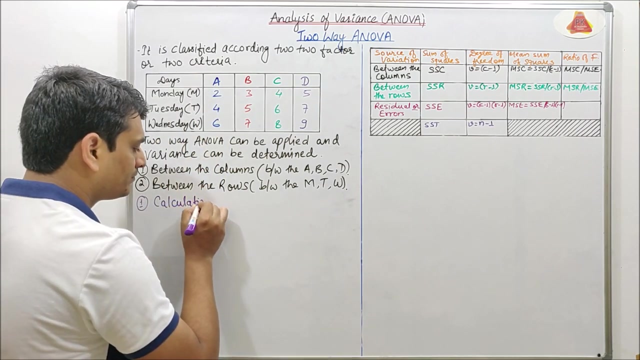 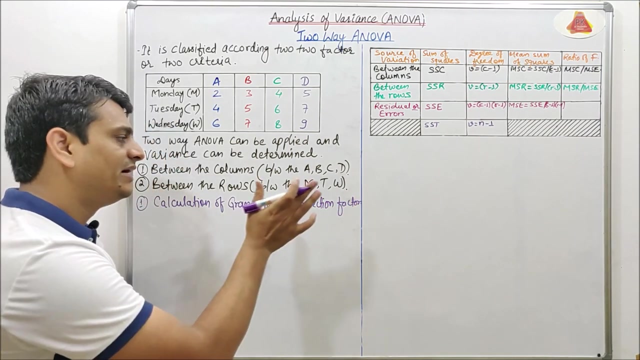 SST is the total sum of square and total degree of freedom. nu is equal to N minus 1.. Now coming to the first step, to calculate two-way ANOVA. so first step is calculation of grand total and the correction factor. For easy calculation of this grand total and the 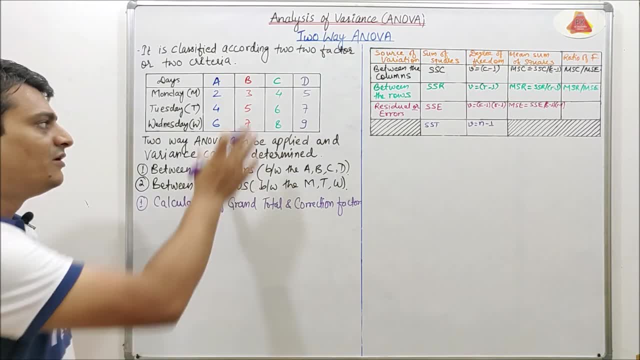 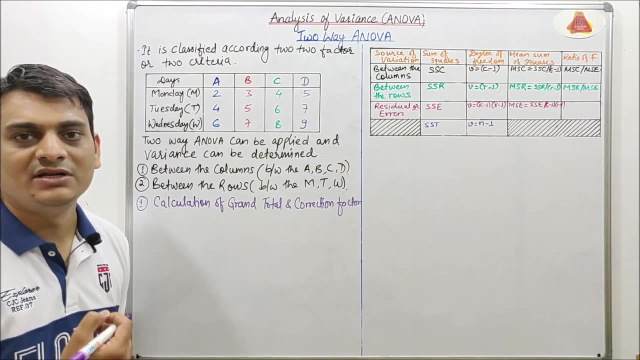 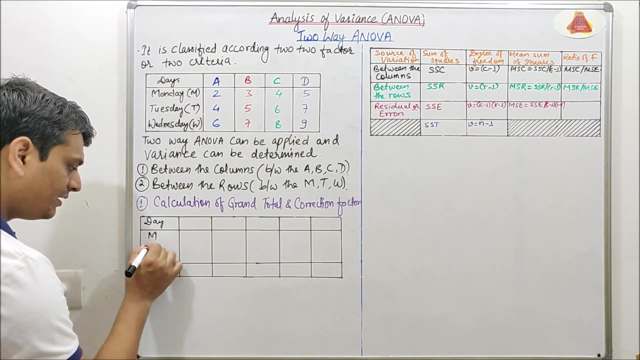 correction factor. let's guess a mid value for this table, and here we are taking 5 as a mid value for easy calculation and the table for calculation will be like this. So this is the table. here we will take. day that is Monday, Tuesday and Wednesday: here we will take: 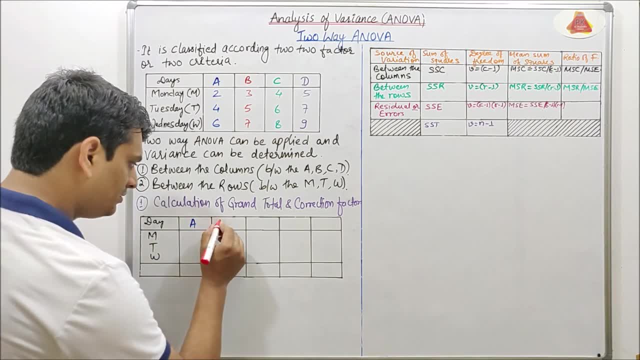 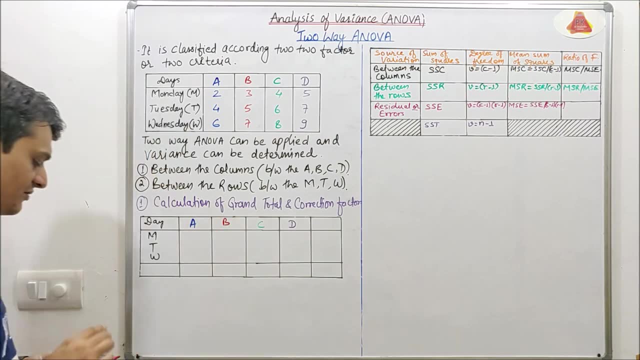 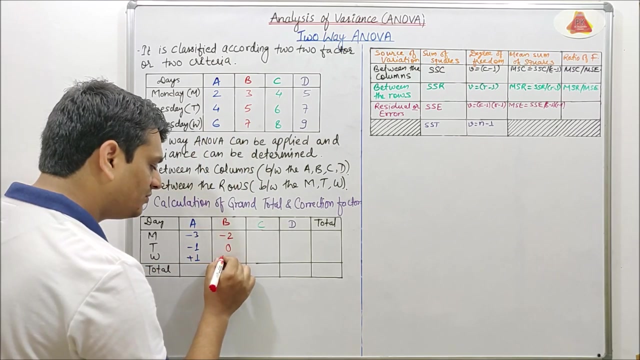 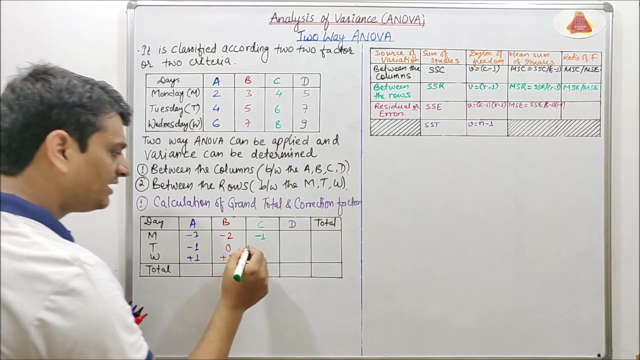 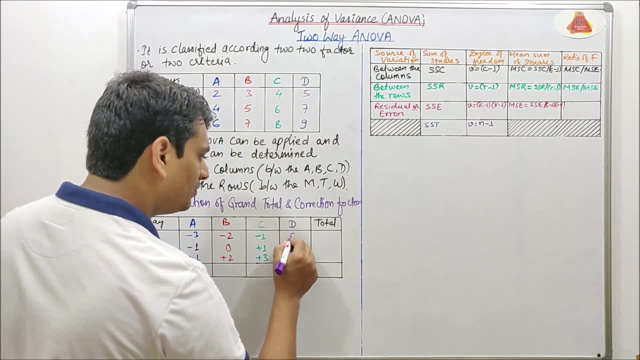 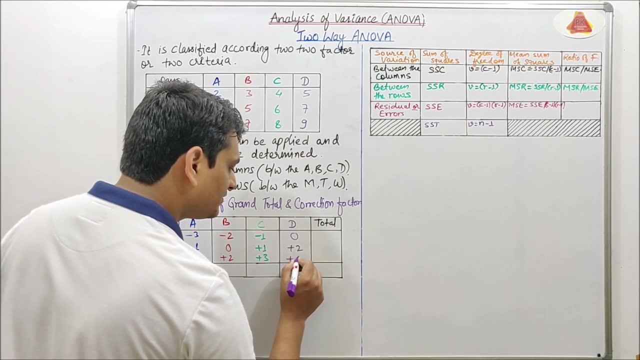 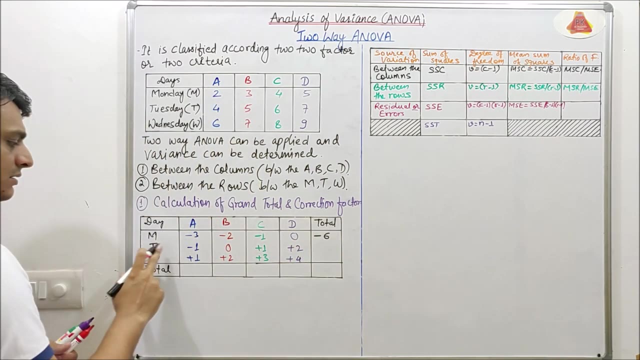 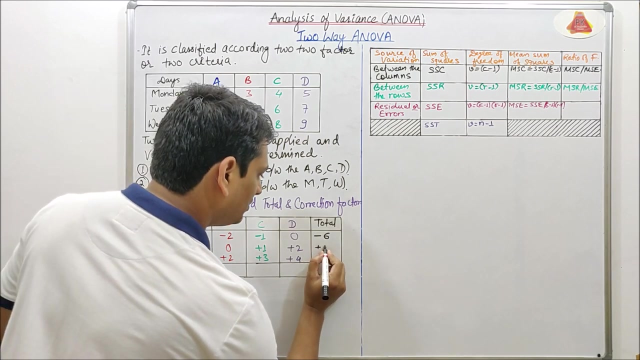 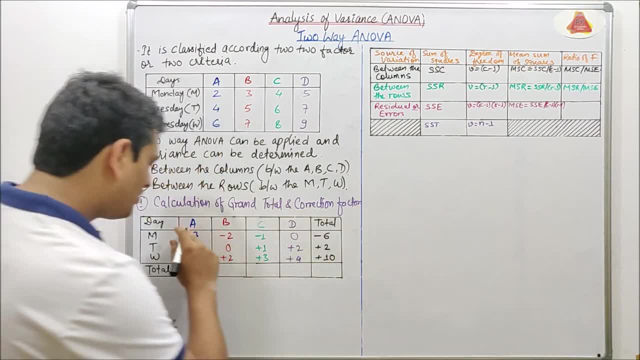 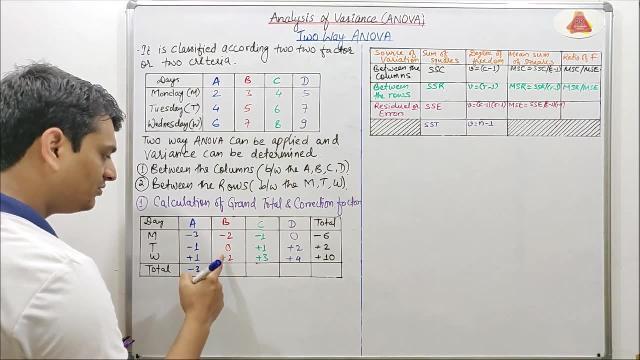 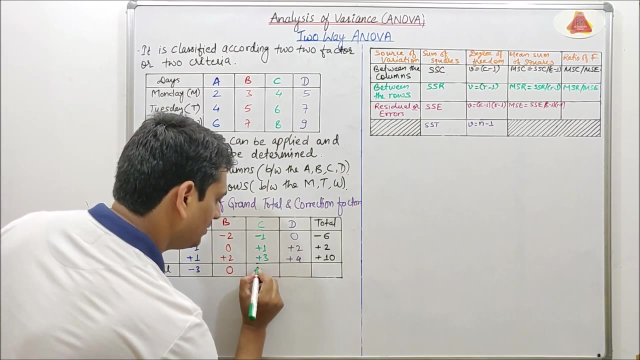 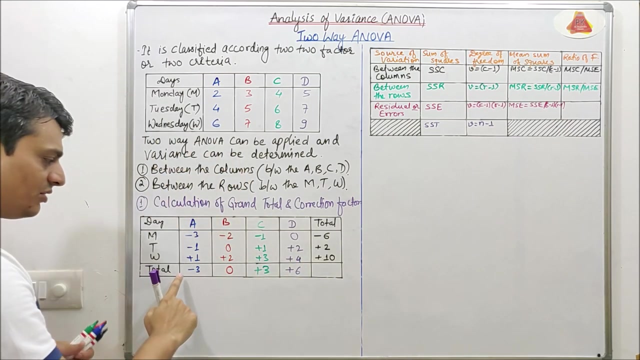 plus 3 plus 4 is equal to plus 10.. now coming to the first column. so here, minus 3 minus 1 plus 1 is equal to minus 3 minus 2. 0 plus 2 is equal to 0. minus 1 plus 1 plus 3 is equal to plus 3, and plus 2 plus 4 is equal to plus 6, and the total of all this value will be minus 3, 0 plus 3 plus 6. 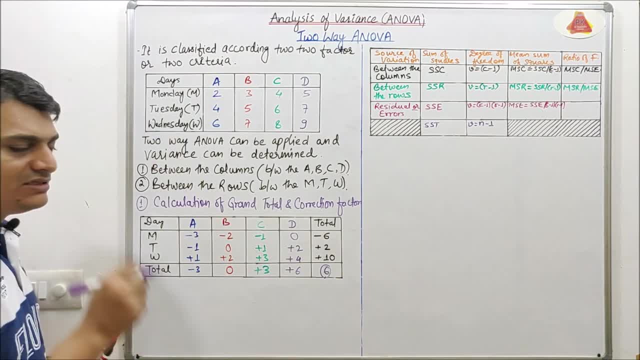 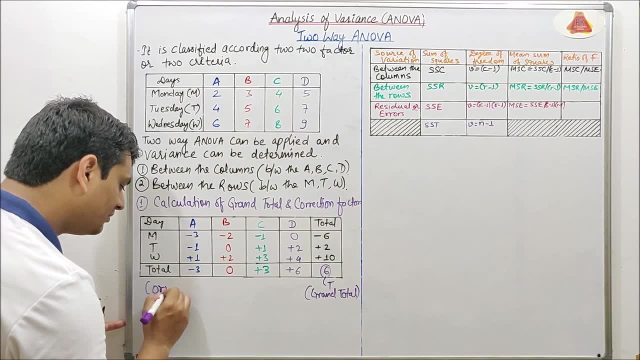 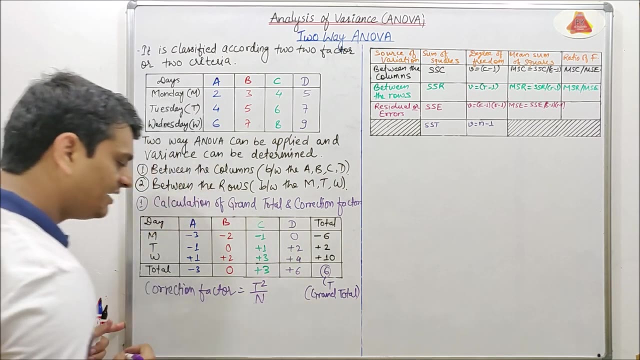 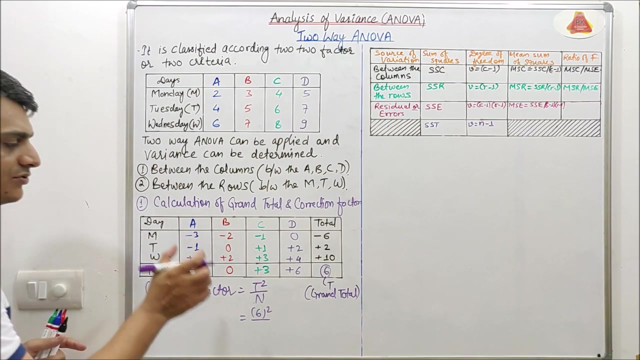 is equal to 6. this 6 is known as grand total and it is denoted by t. now coming to the correction factor. so correction factor is equal to t square divided by capital n. so here t square means 6 square divided by capital n. capital n is equal to total. number of observations. 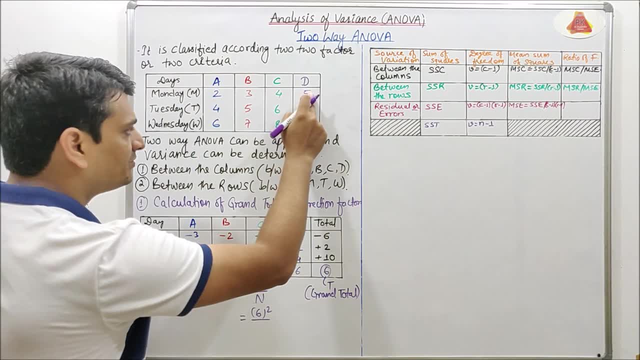 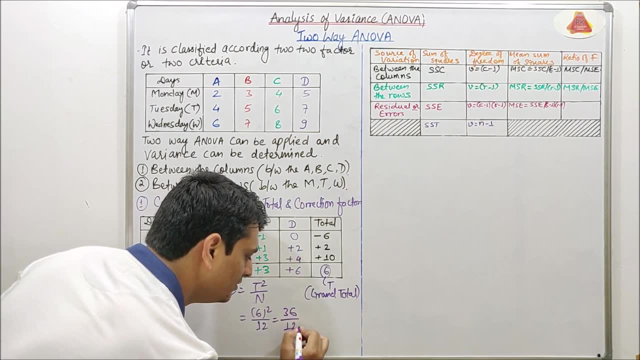 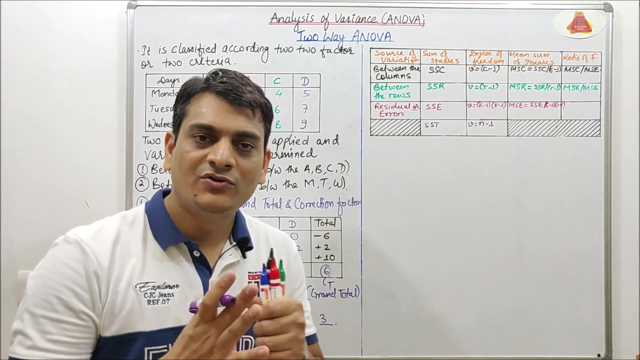 so here, total number of observations are 4 columns are there and 3 rows are there. so 4 into 3 is equal to 12. so it will be 36 by 12. so ultimately, correction factor will be equal to 3. now coming to the second step of two-way ANOVA, and the second step is calculation. 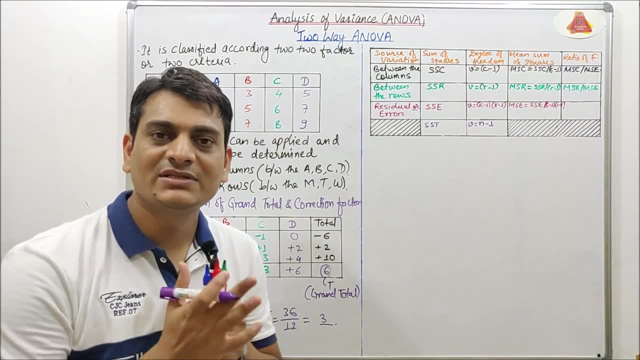 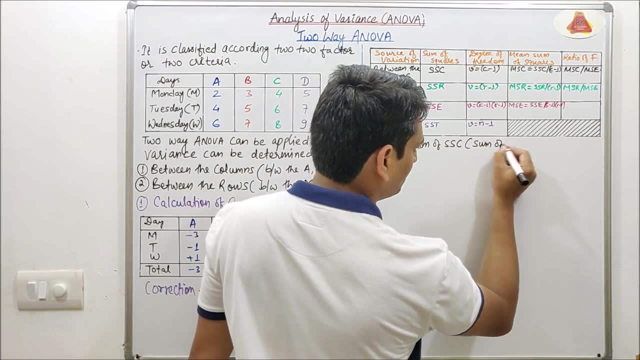 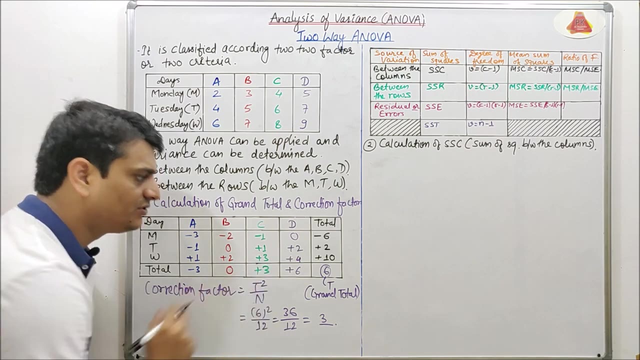 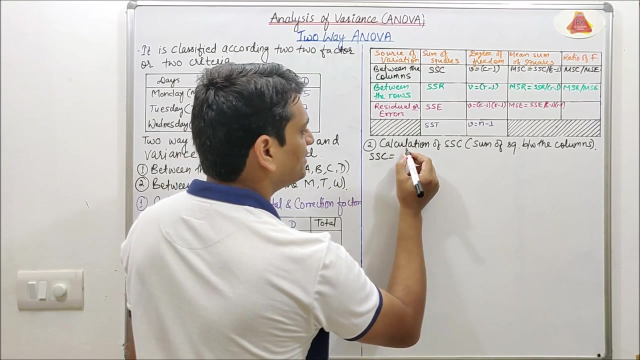 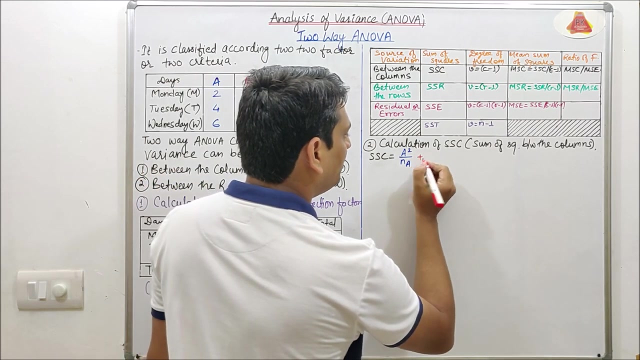 of this ssc, which is calculation of sum of squares between the columns. so this ssc can be calculated by squaring of these column totals divided by number of observations minus correction factor. so ssc is equal to a square divided by n? a plus b square, divided by n? b plus b square divided by a square. 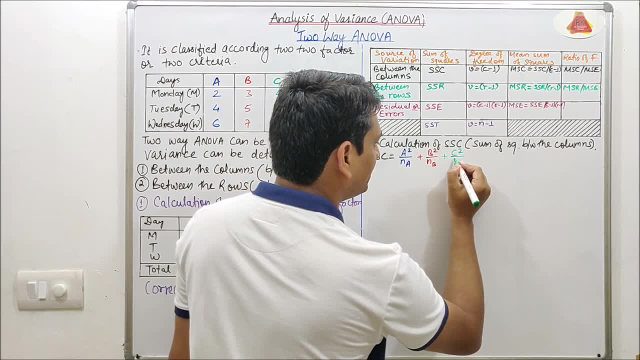 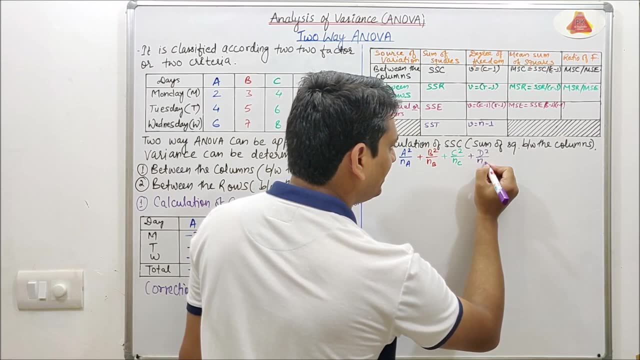 So you can see the ssc I have calculated here. So the ssc I have calculated here. The second step iswriting of the column totals divided by number of observations minus correction: c square divided by nc plus d square divided by nd minus correction factor, that is t square. 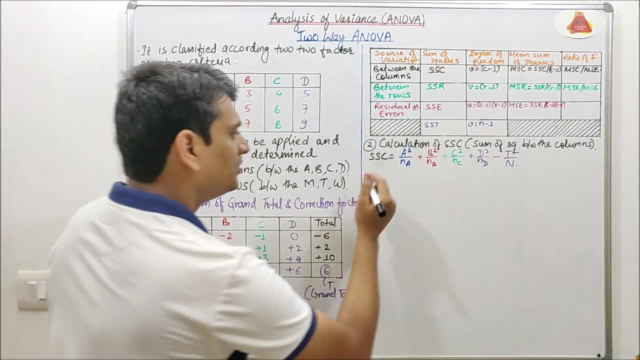 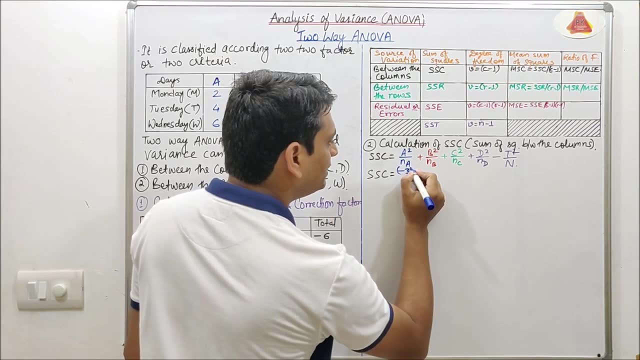 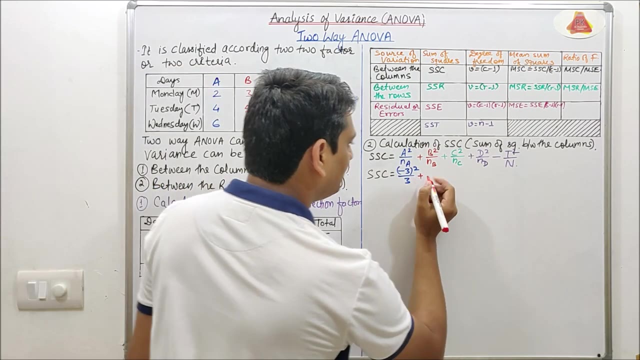 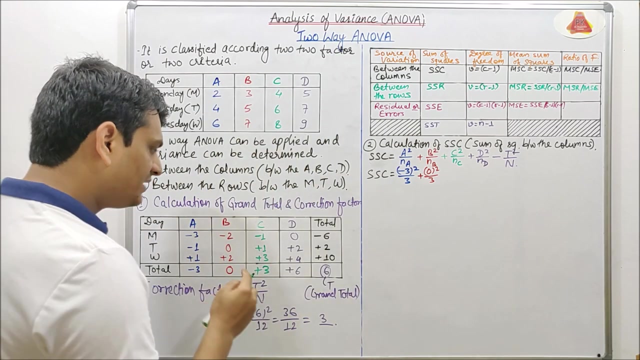 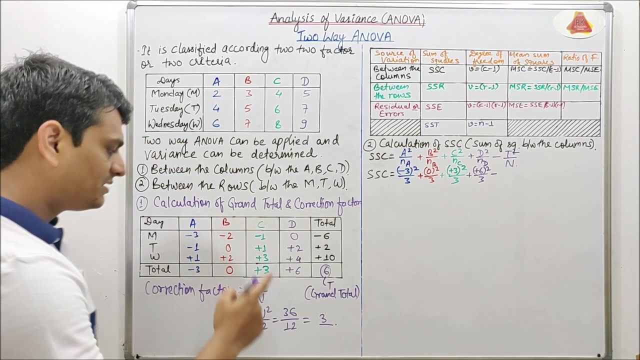 divided by n. so we will put all these values. so ssc is equal to a square which is minus 3 square divided by na, so it is 3. second one is plus 0 square divided by 3 plus plus 3 square divid band by 3 plus plus 6 square divided by three minus. 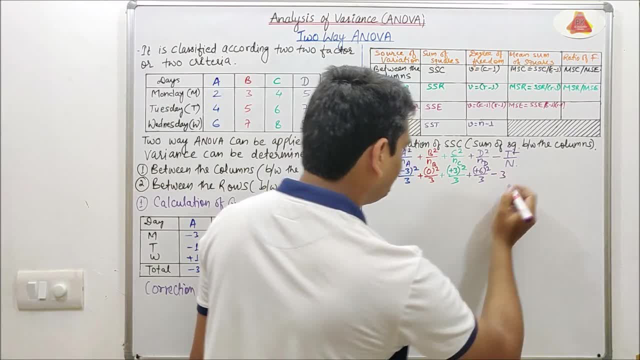 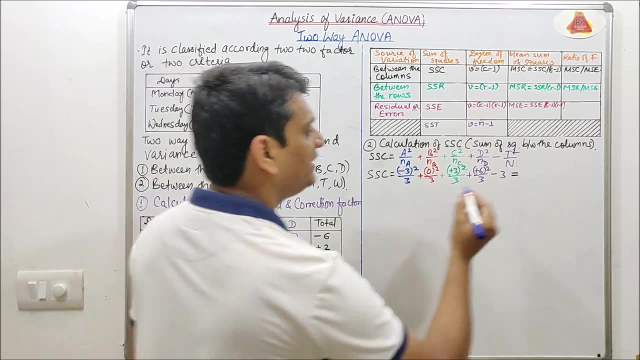 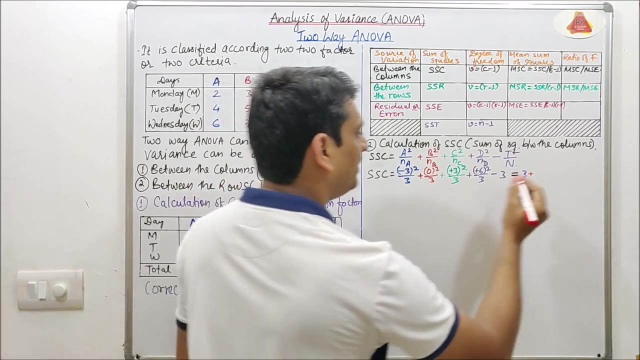 irmi t square by n, which is 3, so it will be equal to minus 3. square is equal to 9. 9 by 3 is equal to 3 plus 0. square is equal to 0. 0 by 3 is equal to 0. 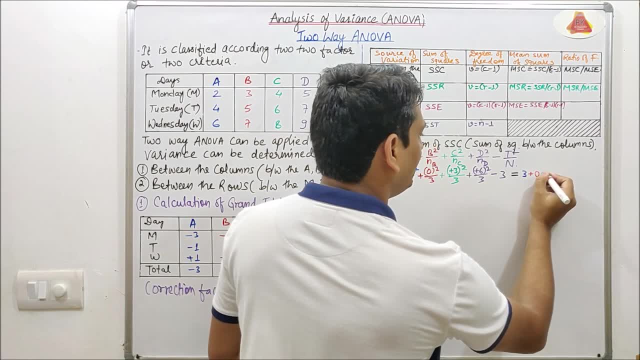 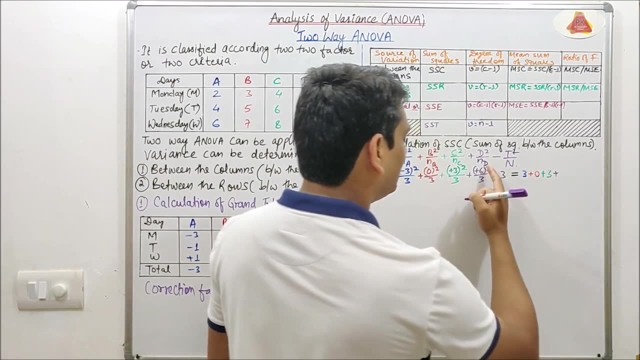 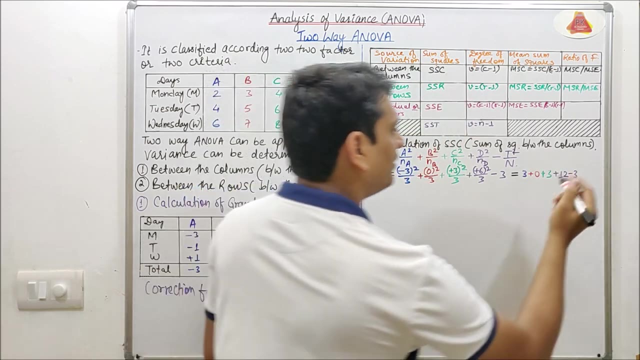 plus 3 square is equal to 9, and 9 by 3 is equal to again, 3 plus 6 square is equal to 36, and 36 divided by 3 is equal to 12 minus 3, so it will be equal to 15. so ssc is equal to 15 because 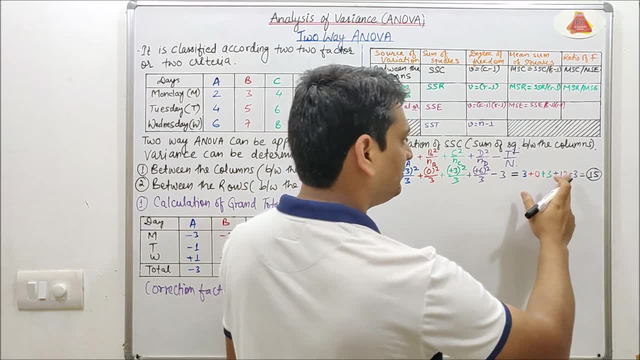 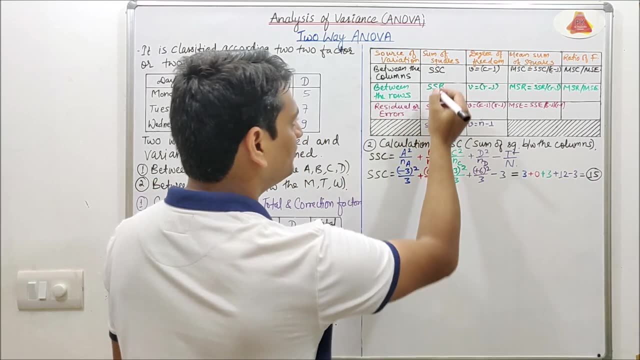 3 plus 0 plus 3 is equal to 6 plus 12 is equal to 18. 18 minus 3 is equal to 15. so ssc is equal to 15, so here it will be equal to 15. nu is equal to. 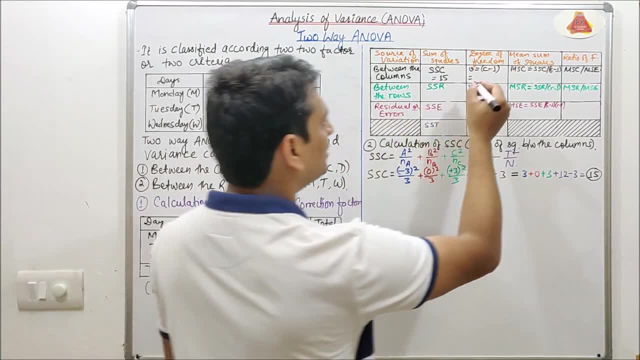 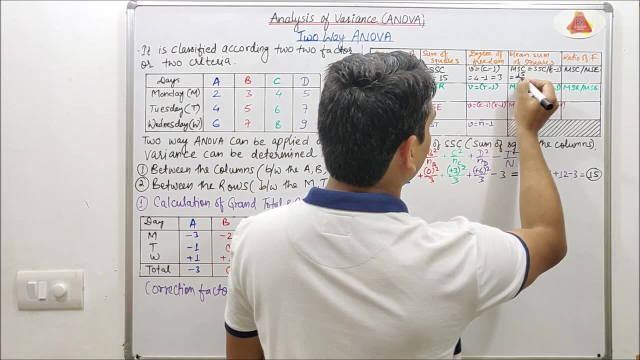 c minus 1. so here 1, 2, 3, 4 columns are present. so 4 minus 1 is equal to 3. so msc is equal to 15 by 3, and 15 by 3 is equal to 5. now coming to the third step of two-way. 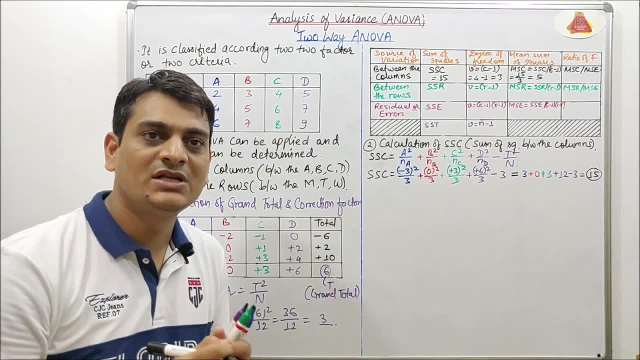 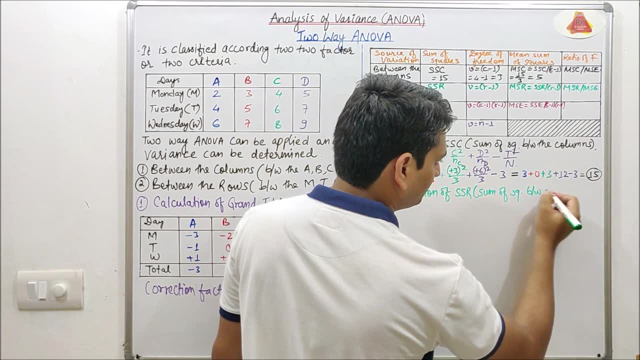 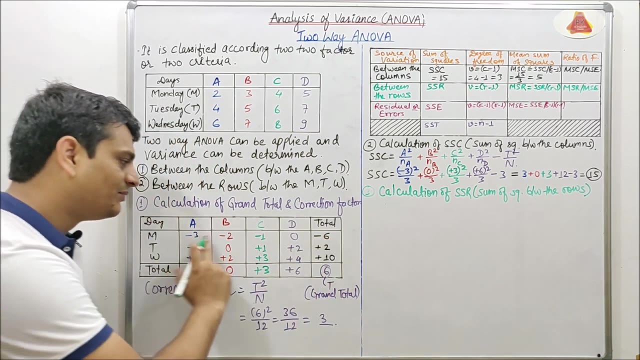 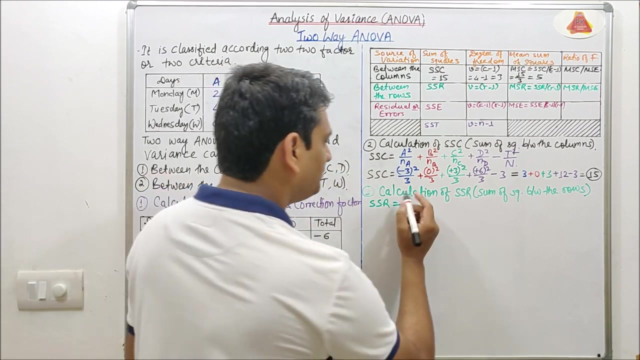 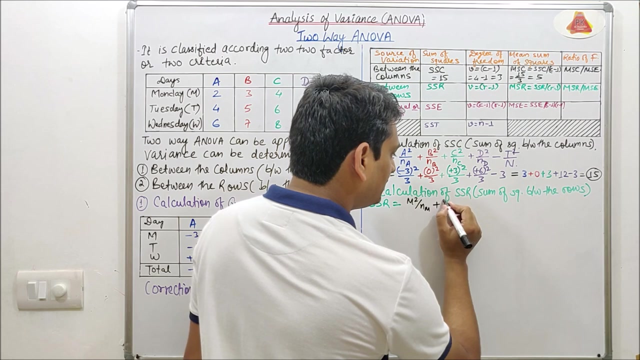 anova, which is calculation of ssr or calculation of sum of square between the rows. so this ssr can be calculated by squaring these row totals divided by number of columns minus correction factor. so ss r is equal to m square by nm plus t square by nt plus. 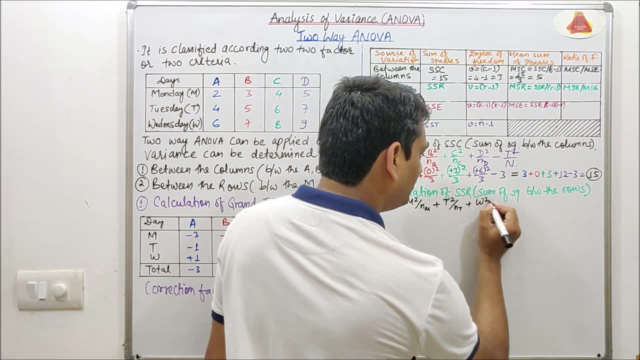 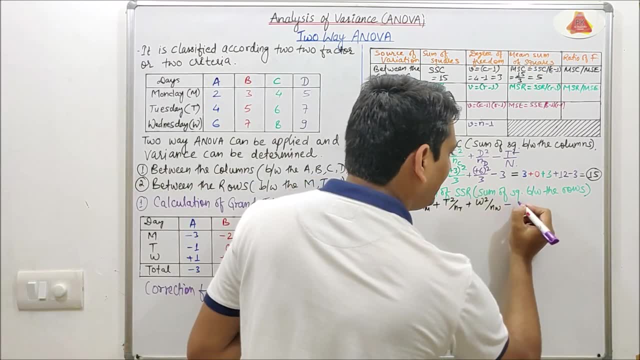 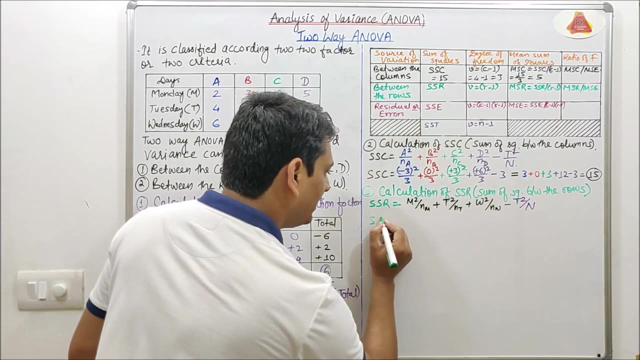 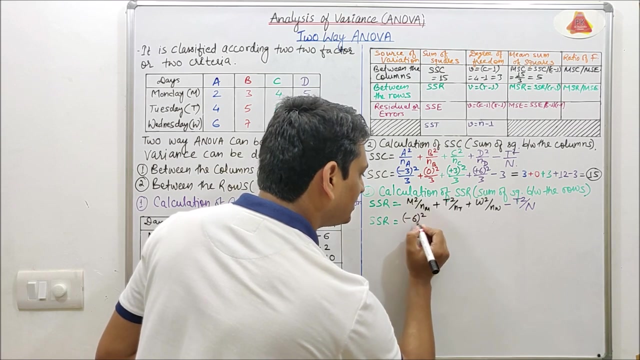 wm square by nt, square by nw, minus correction factor, which is t square divided by n. so it will be t square divided by n. now we will put all these values. so ssr is equal to square of monday row. total that is minus six. so minus six square divided by. 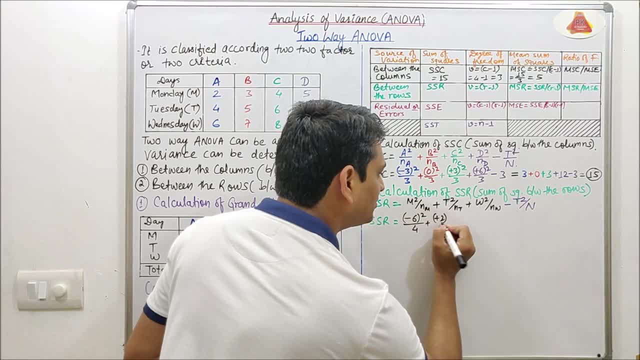 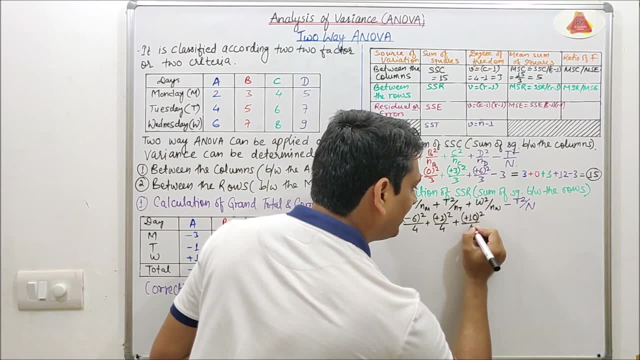 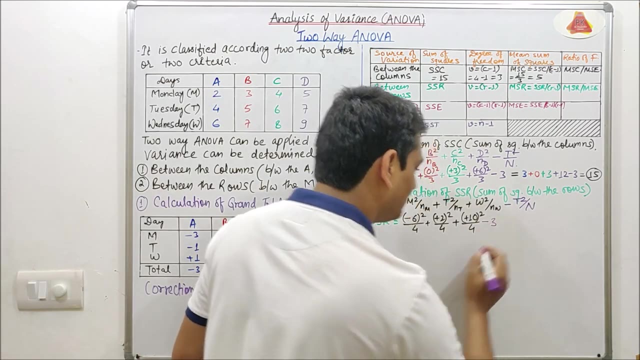 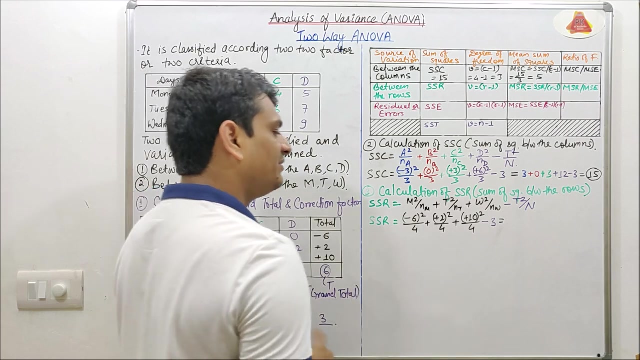 four plus plus two square divided by four plus plus ten square divided by four minus t, square by n, and value of t square by n is equal to three, so it will be equal to minus six. square is equal to thirty six. thirty six divided by four is equal to nine. 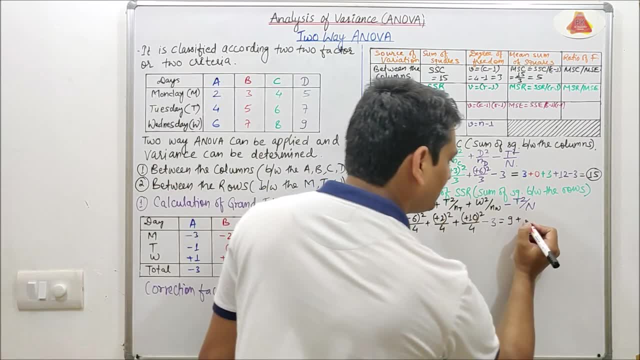 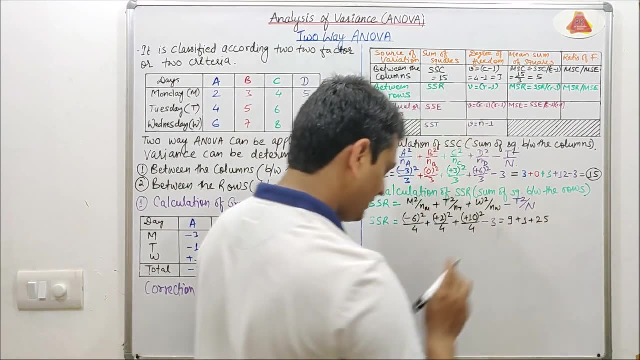 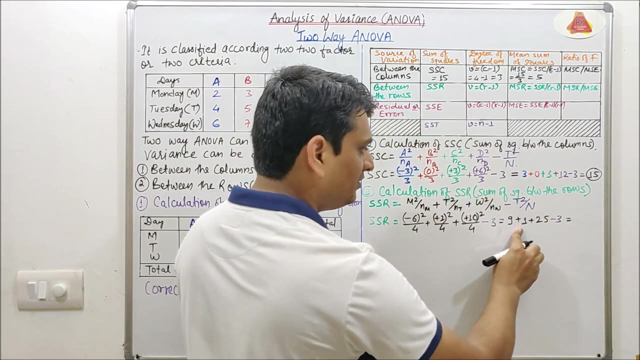 plus plus two square is equal to four. four by four is equal to one plus ten square is equal to hundred. hundred divided by four is equal to twenty five minus three. so it will be: ultimately: nine plus one is equal to ten. ten plus twenty five is equal to thirty five. thirty five minus three is equal to: 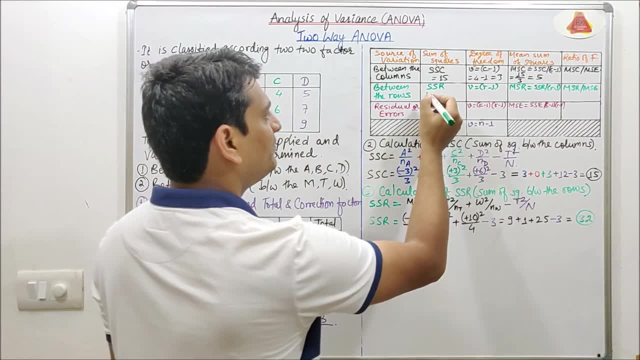 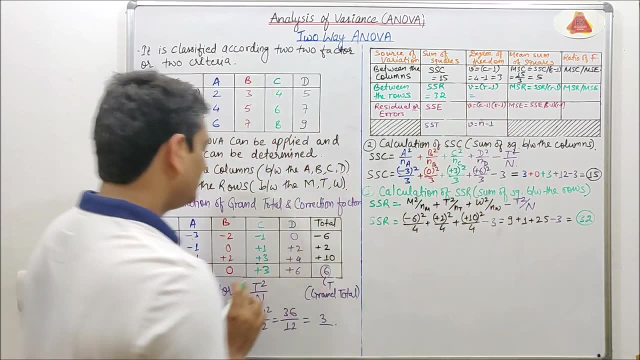 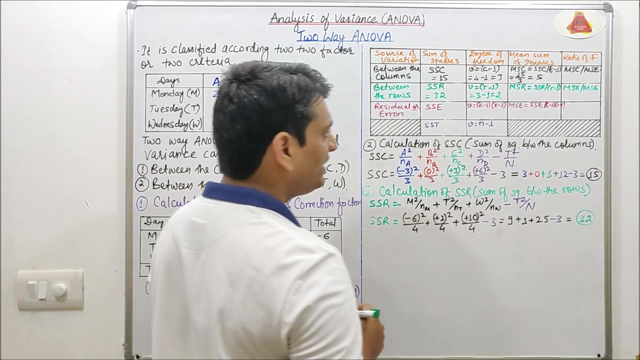 thirty two. so in this table we will put the value of ssr, which is thirty two, and the degree of freedom is equal to r. so r is one, two, three, so it will be three minus one, so it will be two, and the msr is equal to. 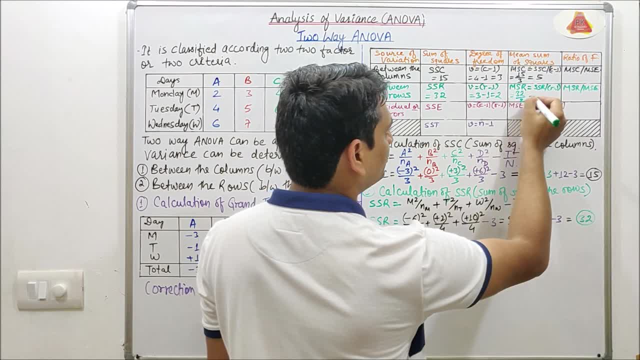 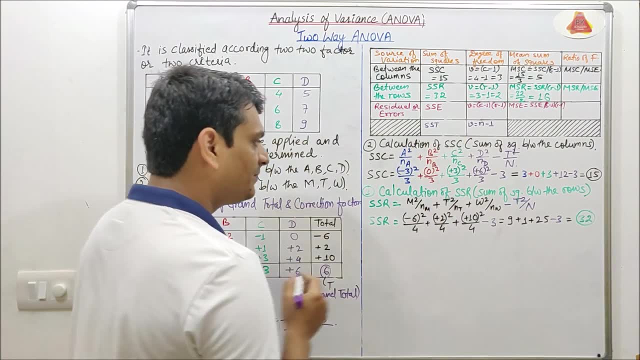 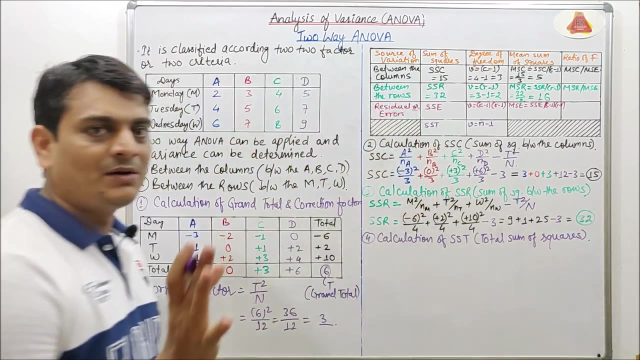 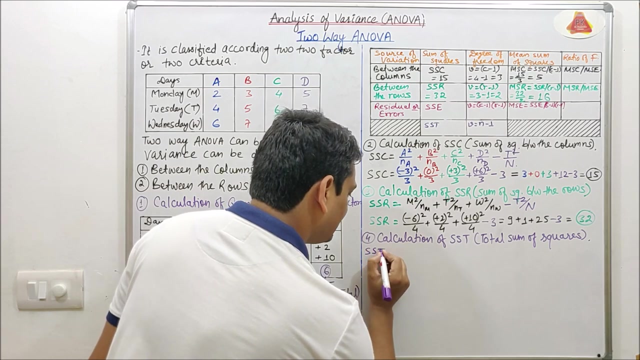 ssr, which is 32 divided by 2, so it will be 16.. now coming to the fourth step, which is calculation of sst, or total sum of squares. so total sum of squares, or sst, can be calculated by squaring all these values. so here sst is equal to. 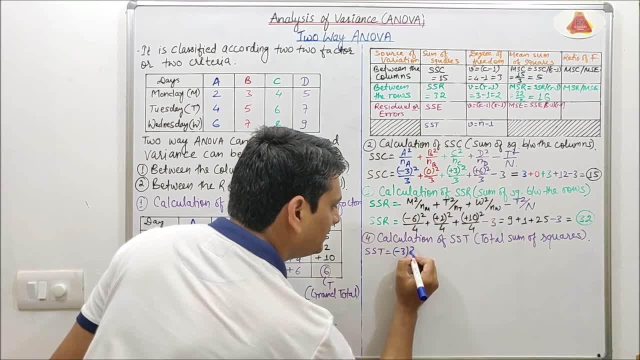 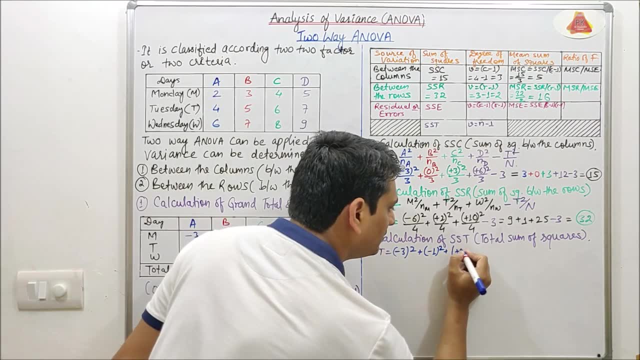 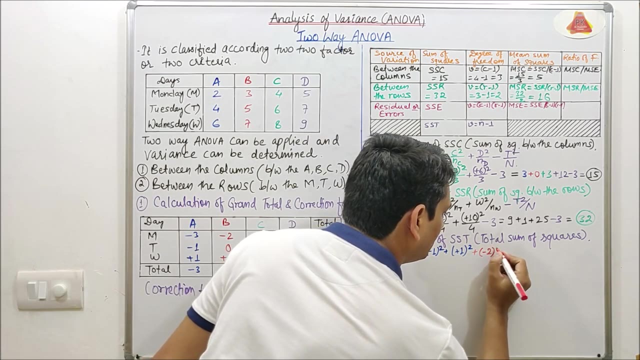 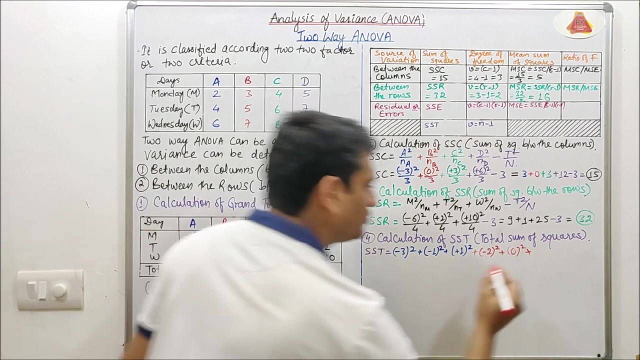 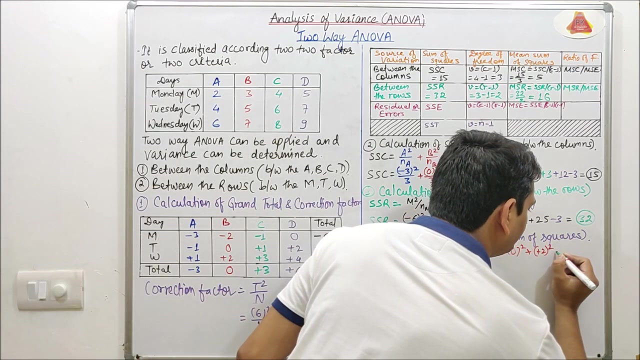 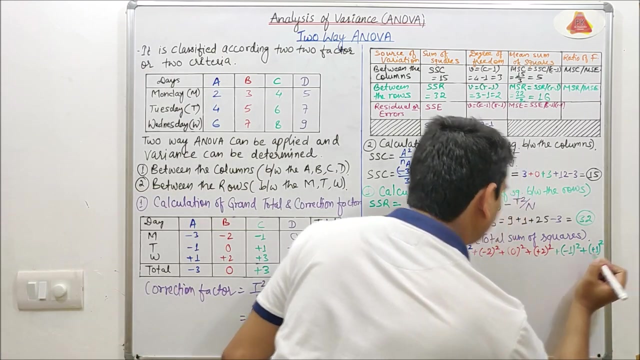 square of minus three plus square of minus one plus square of plus one plus square of minus two plus square of zero plus square of plus two plus square root of minus 1, plus square root of plus 1, plus square root of plus 3, plus. 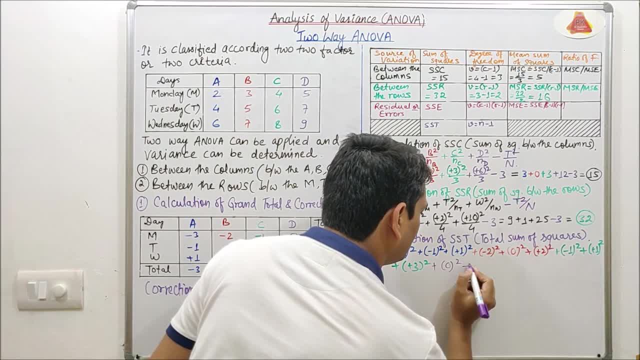 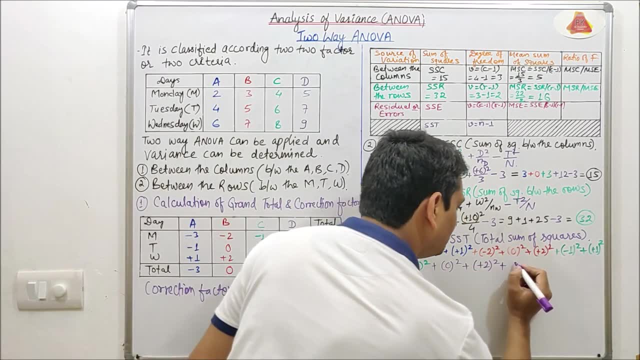 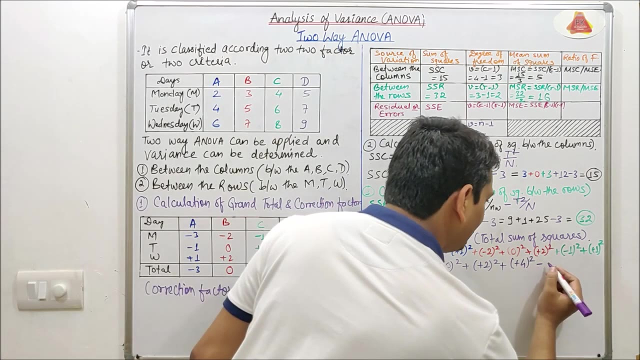 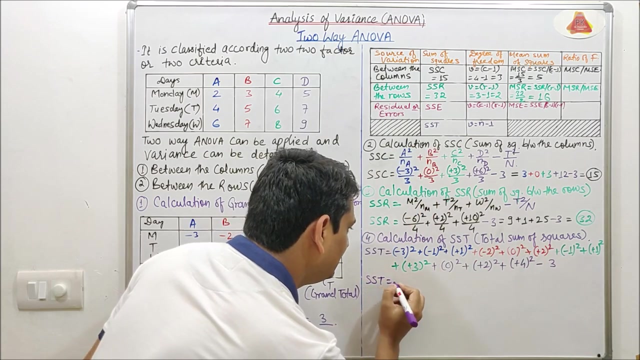 square root of 0, plus square root of plus 2, plus square root of plus 4, minus correction factor, which is t square by n, and t square by n is equal to 3.. So after solving this, we will get: s is t is equal to minus 3, square is equal to 9 plus 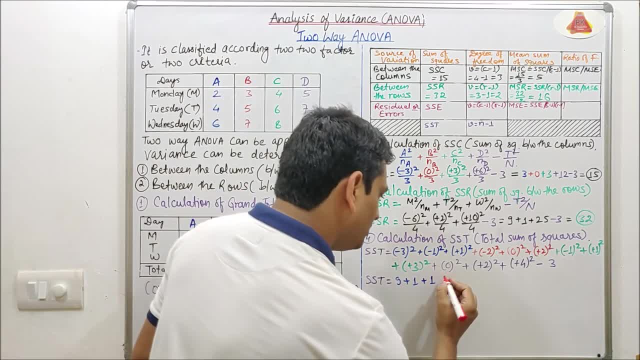 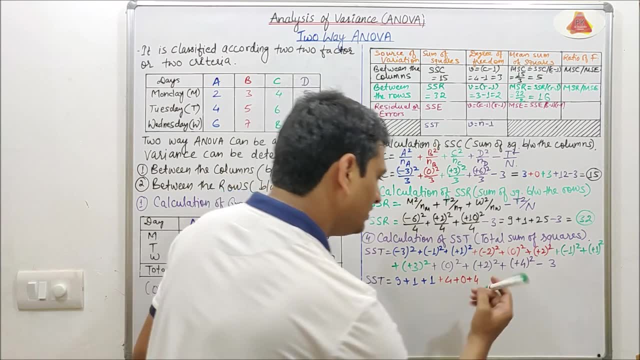 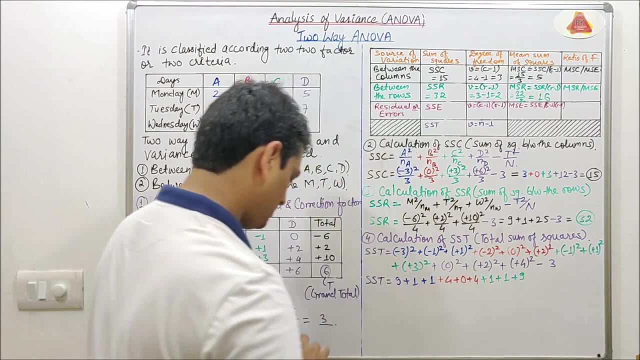 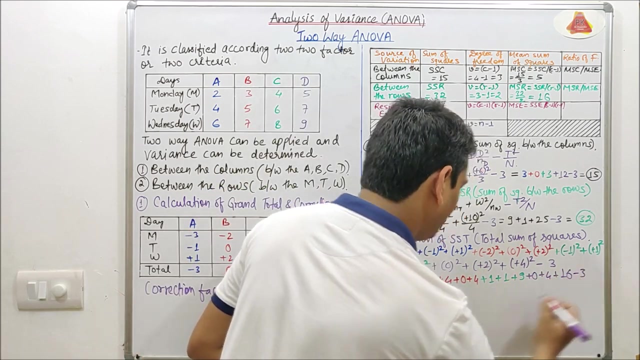 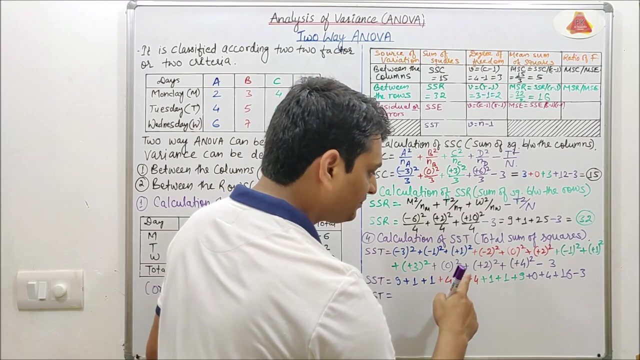 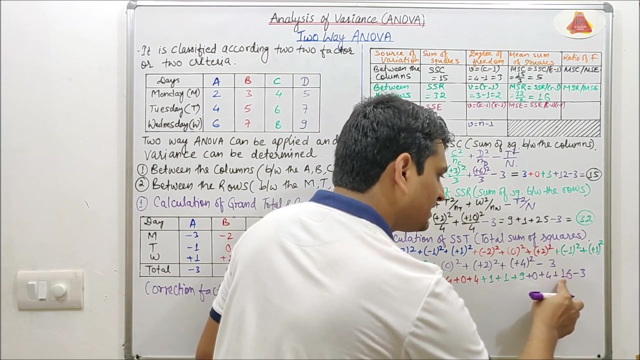 1 plus 3.. 1 plus 4 plus 0, plus again 4 plus 1 plus again 1 plus 9 plus 0 plus 4 plus 16 minus 3, so sst is equal to 9 plus 1, 10, 11, 15, 15, 19, 20, 21, 30, 34, 34 plus 16 is equal to 50, 50 minus. 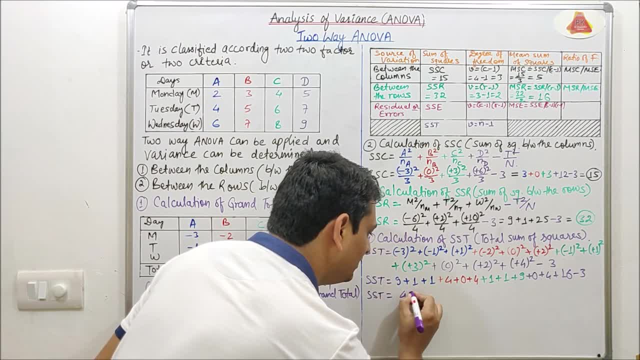 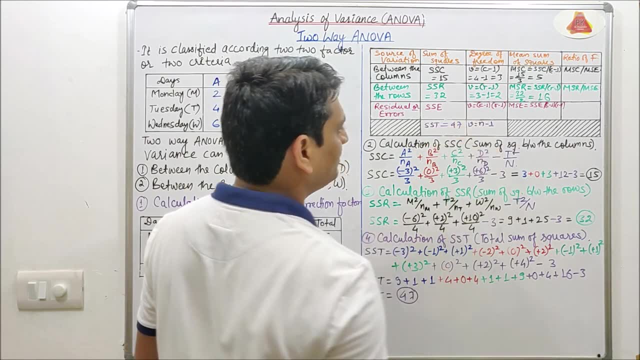 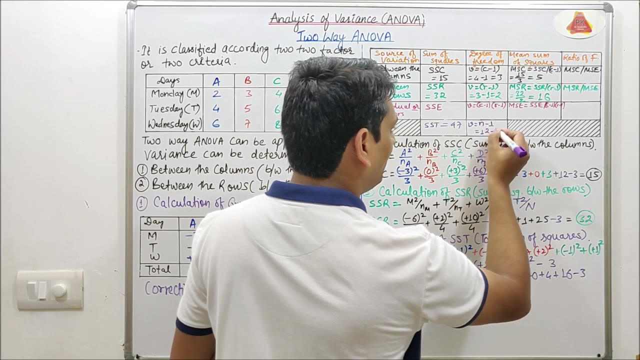 3 is equal to 47, so sst is equal to 47. so here we will put the value of sst, and the sst is equal to 47, and the total degree of freedom is equal to total number of observations, which is 12 minus 1, so it will be 11.. now coming to the next step, which is calculation of sse. 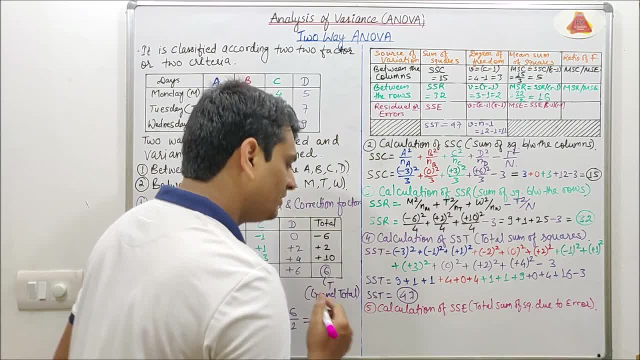 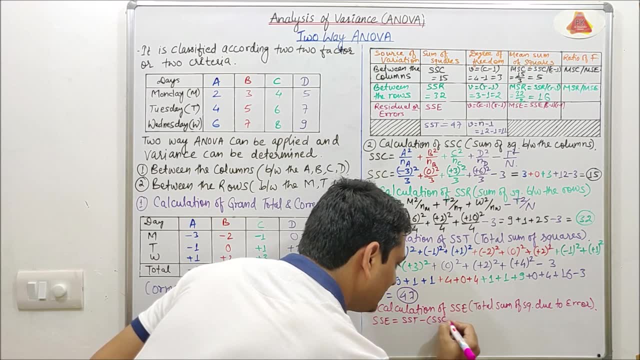 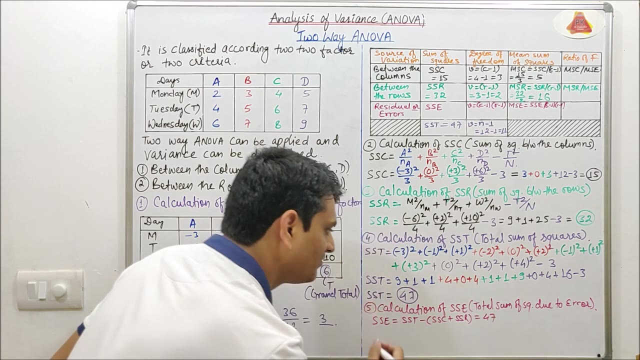 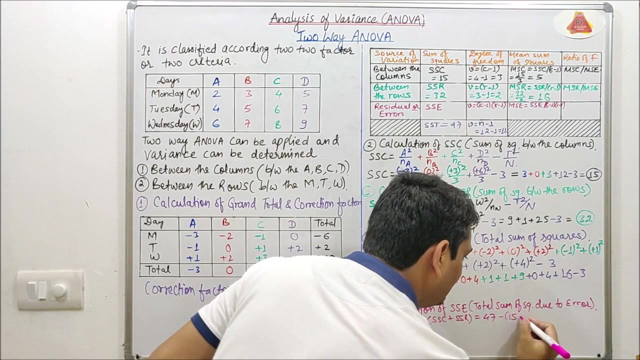 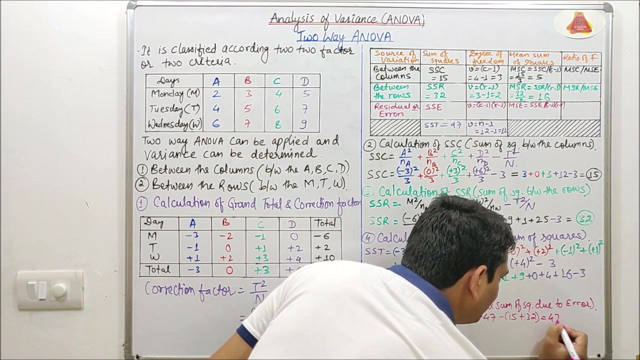 sse is denoted for total sum of square due to error. so sse is equal to sst minus ssc plus ssr, so it will be equal to ssd is equal to 47. 47 minus ssc, which is 15, plus ssr, which is 32, so it will be equal to 47 minus 15 plus 32 is equal to again 47, so it will be zero. 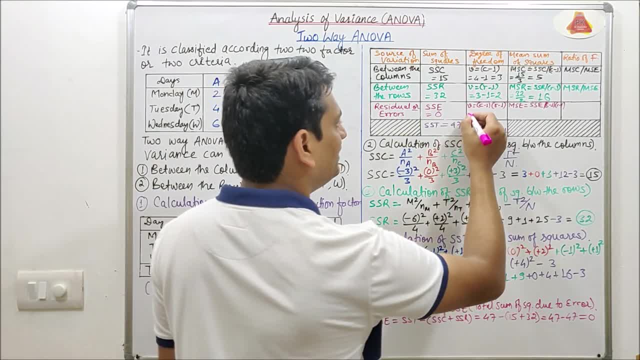 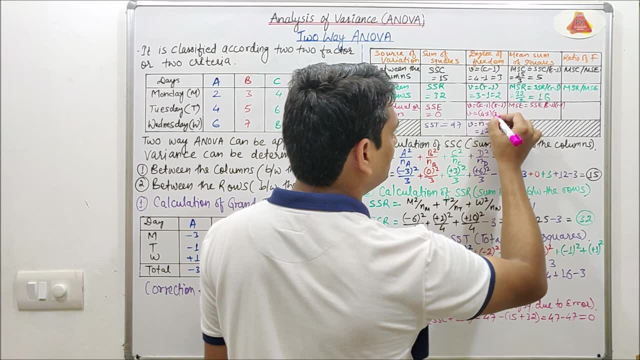 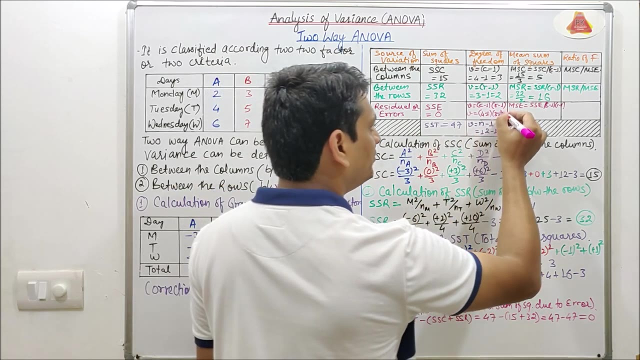 so ssc is equal to zero. so degree of freedom is equal to C minus 1, which is 4 minus 1 into 3 minus 1, so it will be 4 minus 1 is equal to 3 into 3 minus 1 is equal to 2. so 3 into 2 is equal to 6. so MSE is equal to 0 by 6. 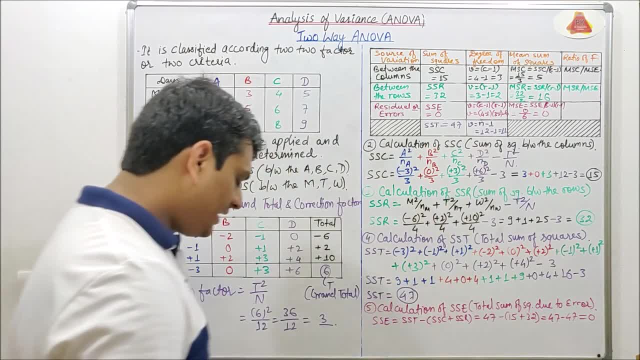 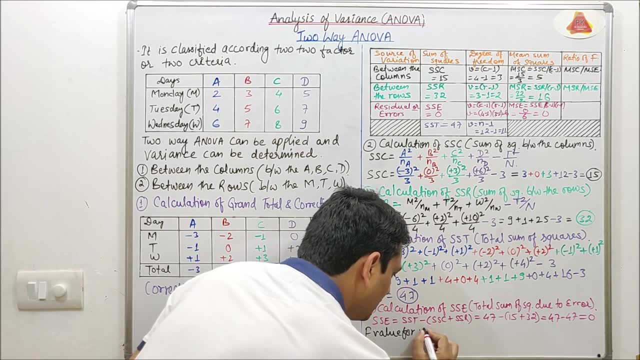 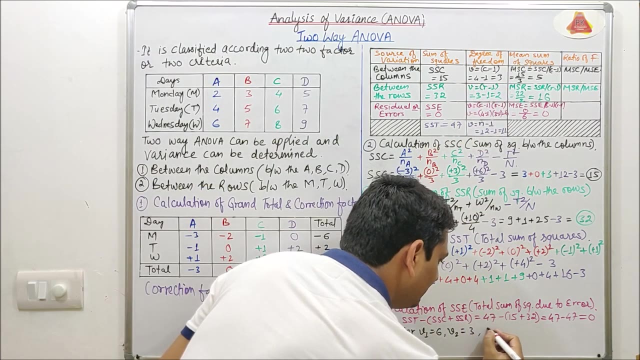 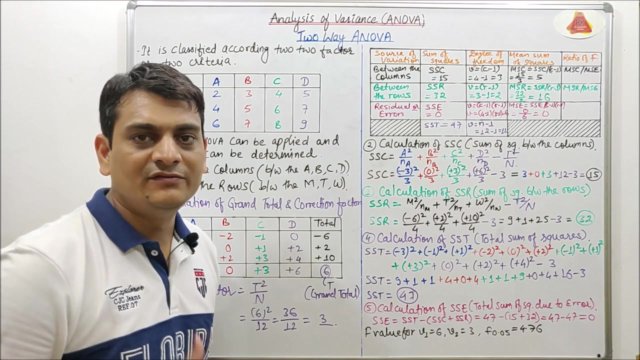 so it will be ultimately 0. now we will take the F value. so F value for new 1 is equal to 6 and a new 2 is equal to 3, so it will be F 0.05 is equal to 4.76, as F table is visible in your screen. 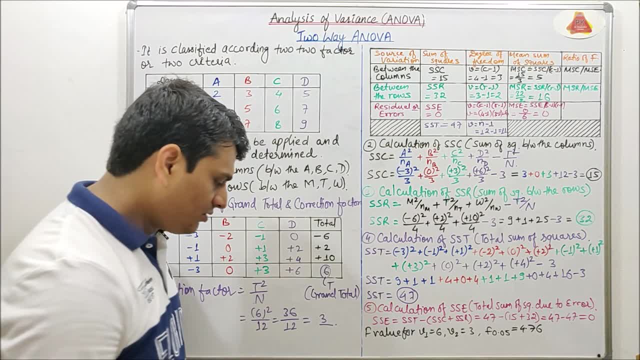 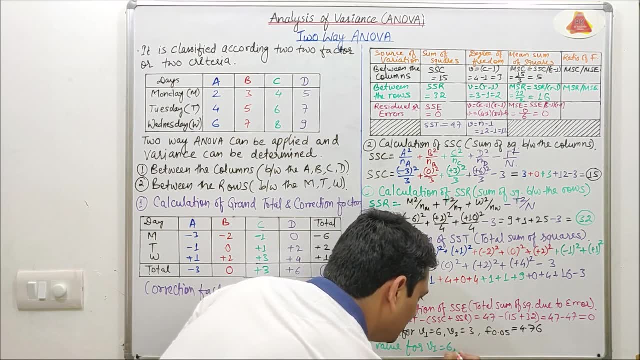 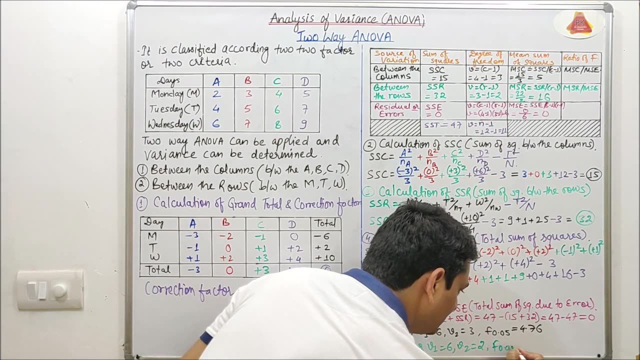 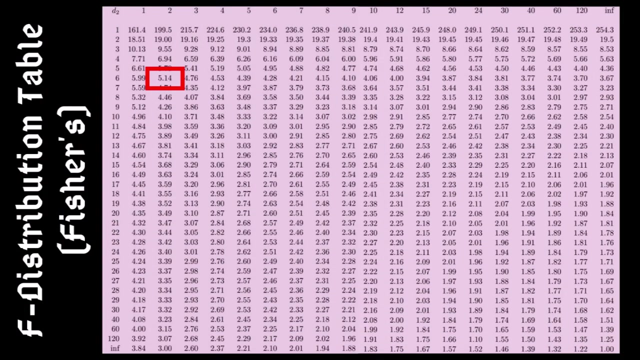 now coming to the next table, the second one, which is F. value for new 1 is equal to, again, 6 and a new 2 is equal to 2, so F 0.05 is equal to 5.14, as it is visible in your screen. 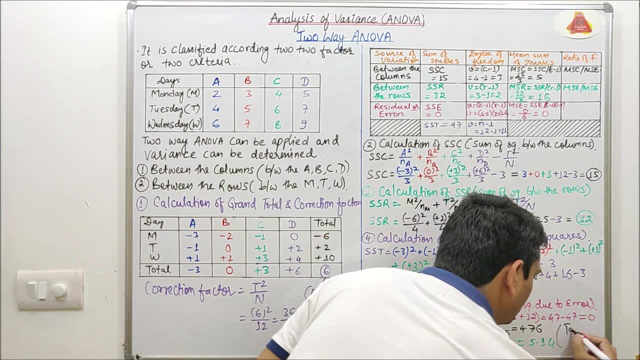 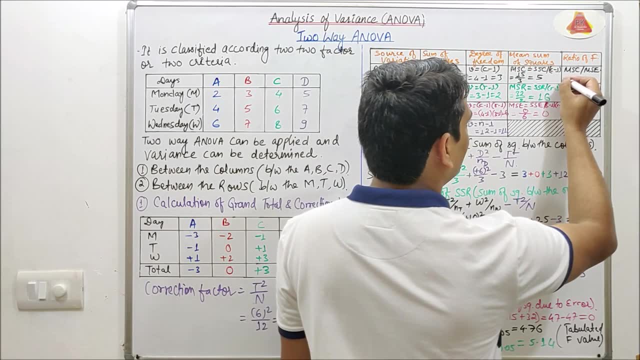 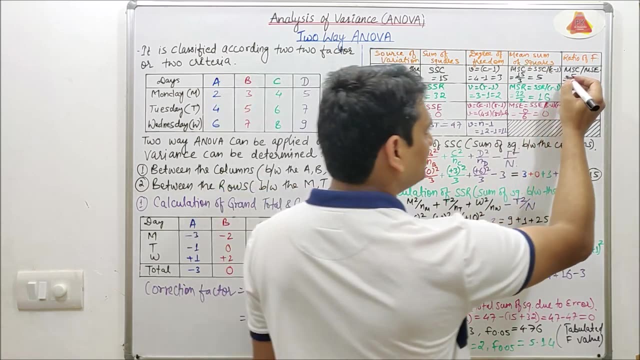 so these are the tabulated F value. now we will calculate the F value for this between the columns. so it will be equal to: MSE is equal to 5 divided by MSE, which is equal to 0. so if we are dividing anything with 0, then it will be. 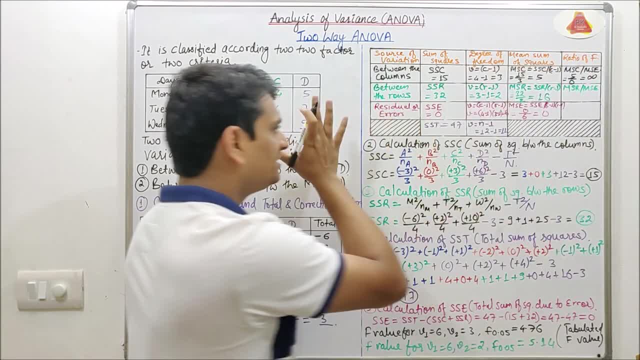 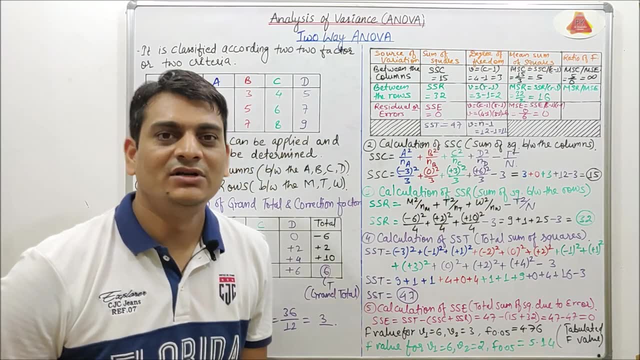 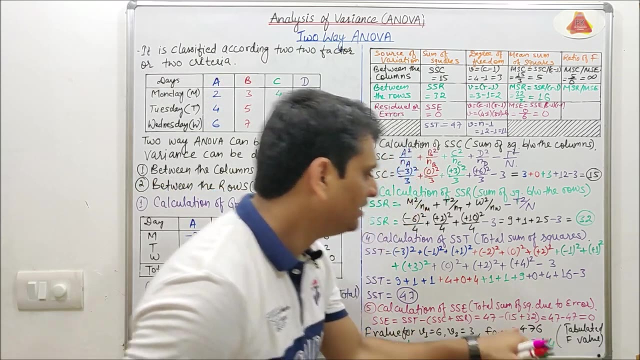 equal to infinite. here in this data we are getting infinite, but generally we will get some number values here. so now we will calculate this calculated F value with this tabulated F value. so tabulated a value is 4.76 and a calculated value is greater than this 4.76, it means there is 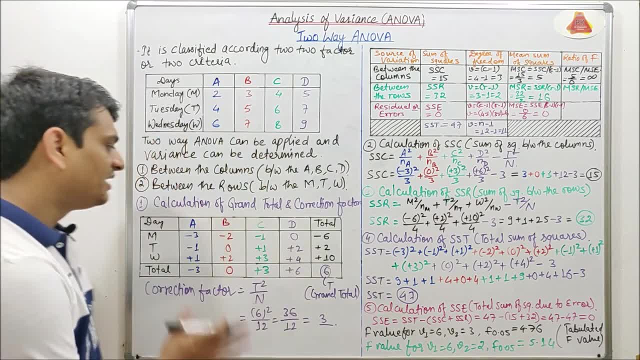 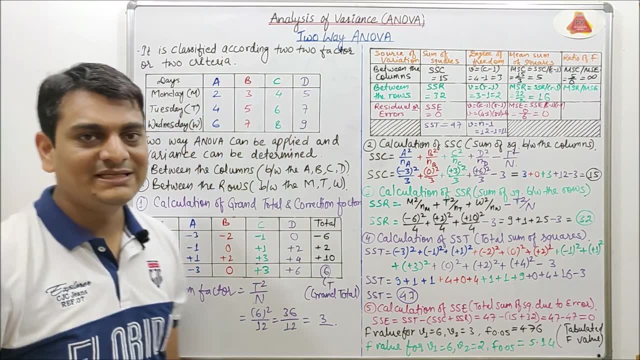 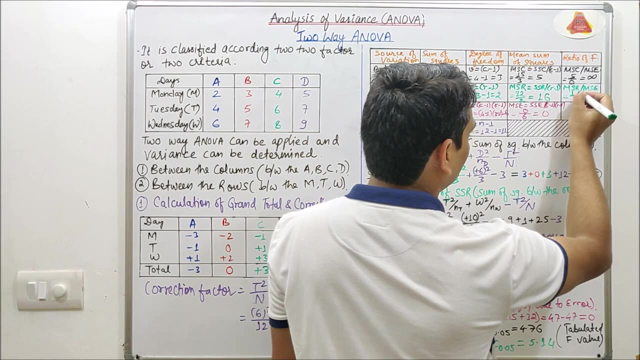 significant difference between the students which are a, b, c and d. so there is significant difference between the study hours amongst all these students. now coming to the second one, which is between the rows, a value for between the rows. so it will be equal to 16. that is value of msr divided by mse. 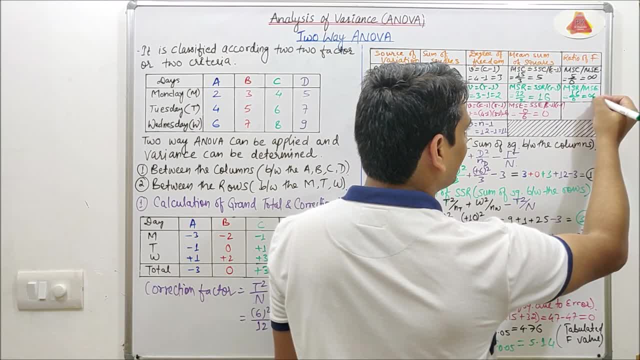 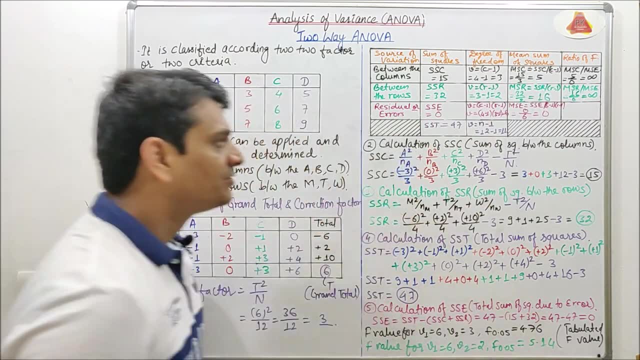 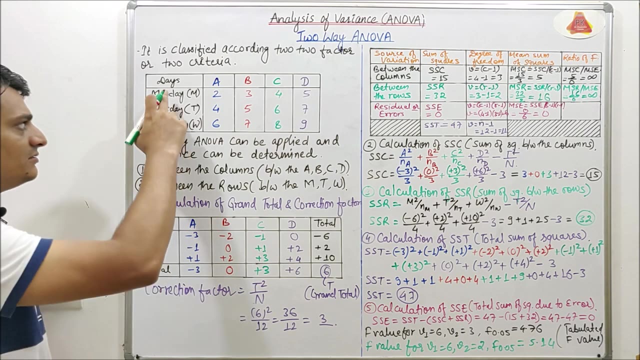 that is again 0. so after calculation it will be again infinite. so here also, calculated value is infinite and tabulated value is 5.14. so calculated value is greater than the tabulated value. it means there is significant difference amongst these days means in monday, tuesday and wednesday. so here we.